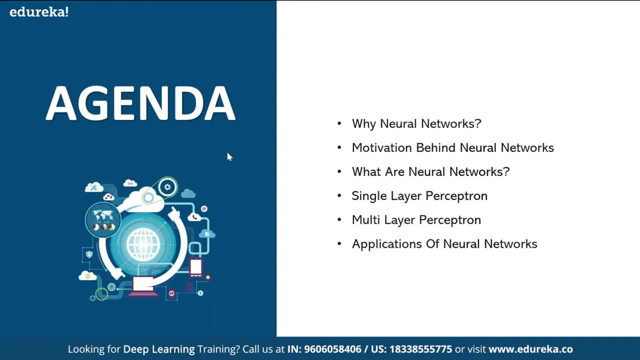 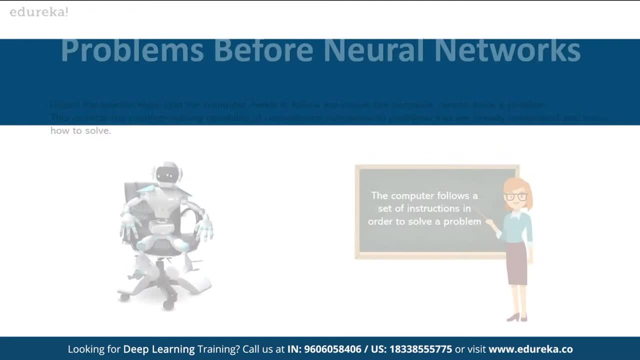 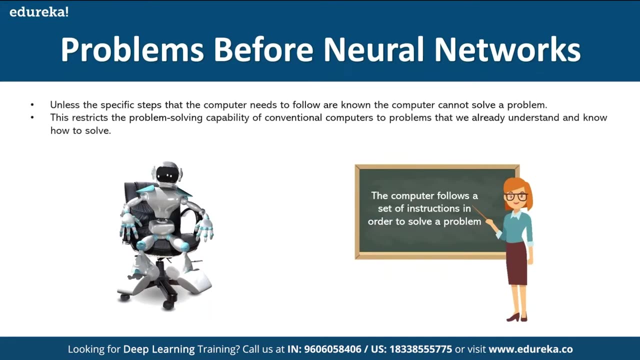 we'll end the session by understanding what are the applications of neural network. Okay, so let's start the session. Why neural networks? So, as I said, we are trying to mimic the human brain, right? How can we do that? So for that, we require an algorithm Now. 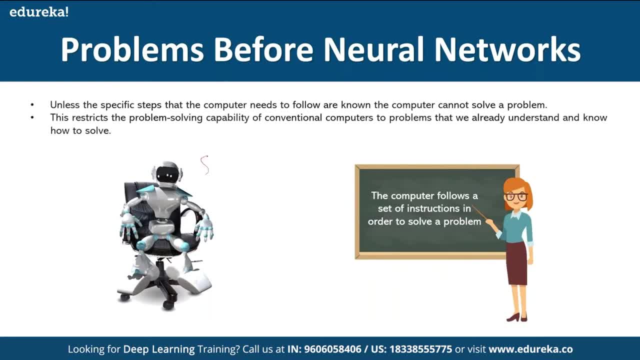 these algorithms are fed into the brain of a robot. Okay, in today's world, we have Alexa, we have Google assistants- right? All these require some programs or algorithms to take actions. Okay, so these set of instructions are required for the robot to take actions. right, So these can be accomplished using 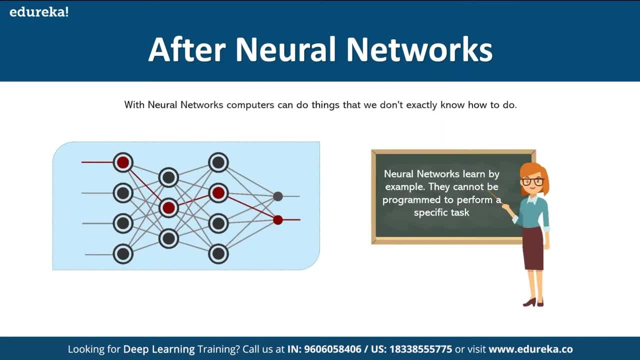 neural networks. So, for example, once- this is how you know- we are going to develop neural networks and these neural networks are going to be trained. We are going to train just like how human brains are trained- right, We are going to train something known as neural 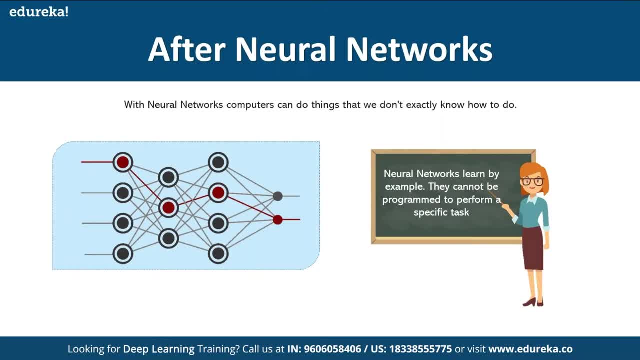 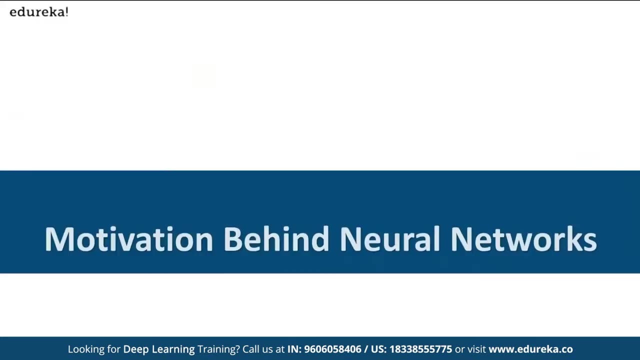 networks post that this neural network will be deployed in the robot's mind and it will be able to follow some specific task. Okay, how it is, what are neurons, what are neural networks? we will understand in detail, but this is just the background of it. So what? 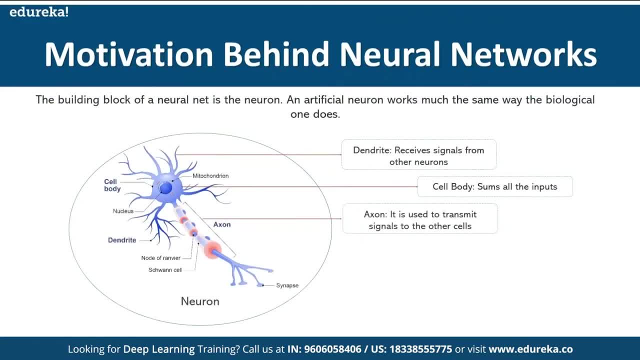 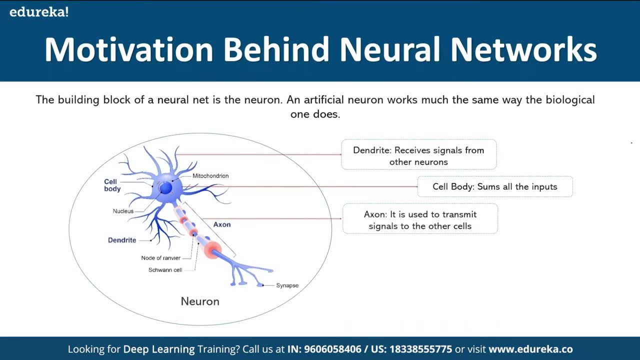 is the motivation behind neural networks. As I said, the human brain is going to be trained, right? So the building block of any human brain is a neuron. right So it is neurons that is the building block of any human brain. So this is how a neuron looks like. So if 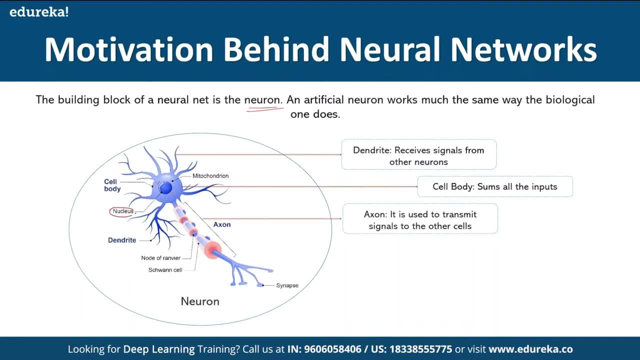 you see it has a nucleus, okay, And you know it has something known as exon, Okay, And these are known as dendrites, Okay. So if you see a dendrite, what they do? they receive. so what happens in human brain? this is suppose this. this represents this image. 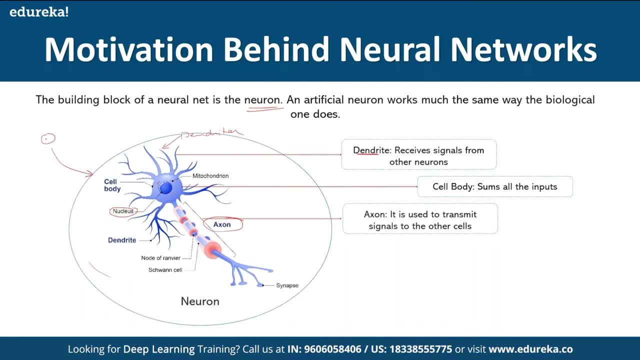 this circle represents this image. Just imagine, inside this, we have this. okay, Now this is connected to another. this, that is neurons. So there are neurons connected with other neurons, So there is a network of neurons. Okay, These are connected with each other. How are they connected? They are connected using 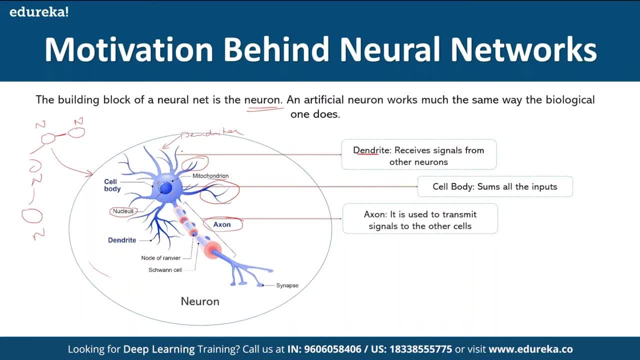 these dendrites. Okay, Now, once they receive an input, right, Once they receive an input from these dendrites, they will process it in that nucleus or the cell body and they will give a output using the exon. Okay, So, for example, suppose we listen to music, right? 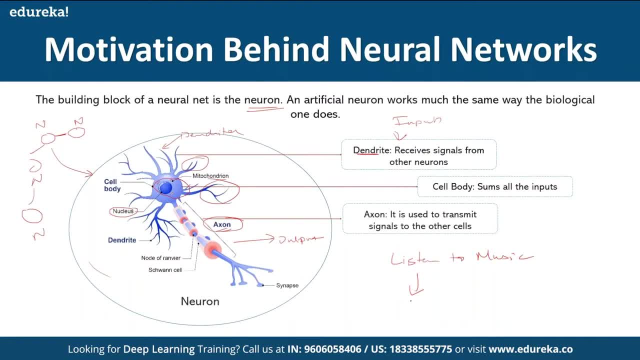 Human. So we listen to music. what happens? Certain emotions are evoked, right, Certain emotions are evoked. So the input to our brain is music right From our ears, So maybe yours are our senses, From that. we listen to music. the neurons, artificial neurons, sorry, the neurons- 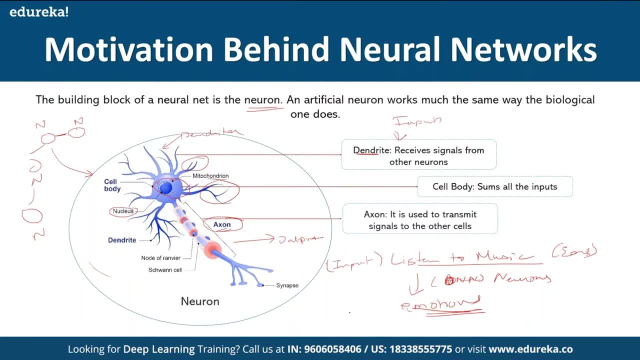 they will process it And your mind will feel the emotions. Your body will feel the emotions right, taking this input for you. the neurons are taking the input, and who? what is it giving you? it is giving you output. each neuron is connected to other neurons, and one and second is each neuron. 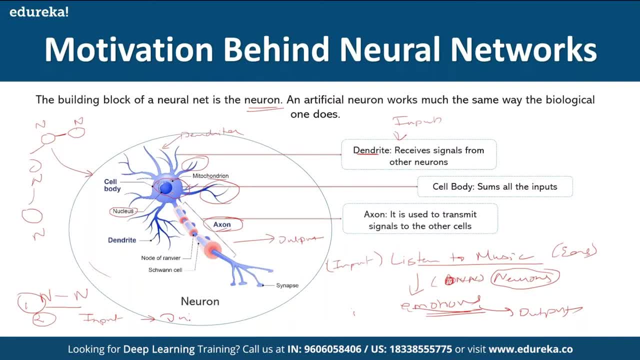 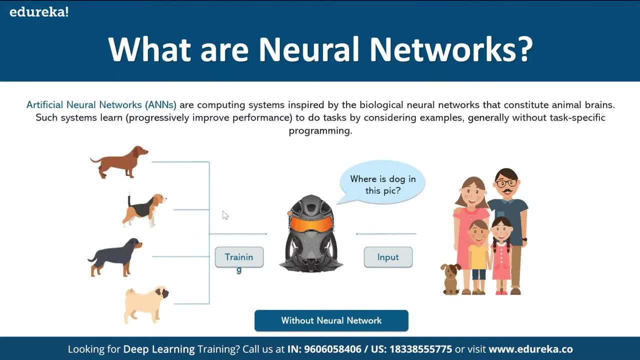 receives the input and it gives the output. so what are neural networks? as i said, like the human brain, what we will do, we will also train our, our we like how our mind remembers, right? so if you hear my voice now, and next time you hear my voice again, right, you will be able to identify it. so, somewhere, 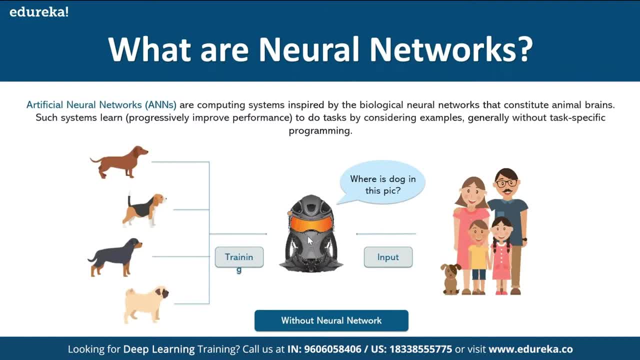 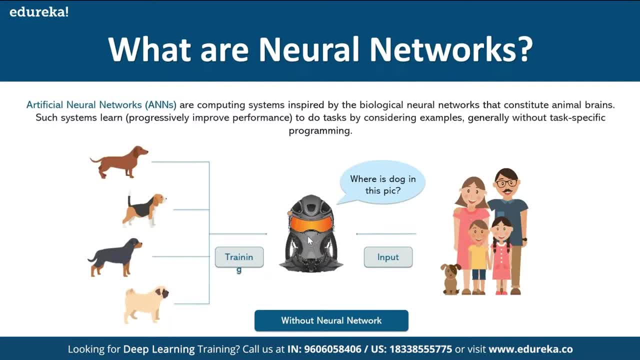 is my father right. So you have trained your mind to understand different relationships, different persons, different concepts, different voices. even smell can make you identify Similarly here. what we are trying to show you here is if your mind doesn't have neurons. 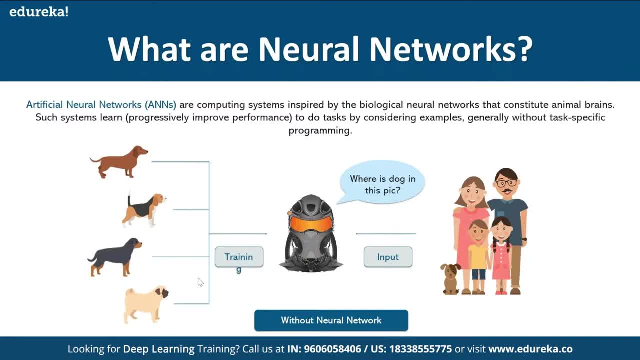 and suppose you see some human beings, right, but you are only seeing the dogs, you're not seeing the other parts. Why? Because your mind has not been trained right. So if you see, if I ask the robot, where is the dog in this pic? Where is the dog in this pic? So suppose you see a mobile. 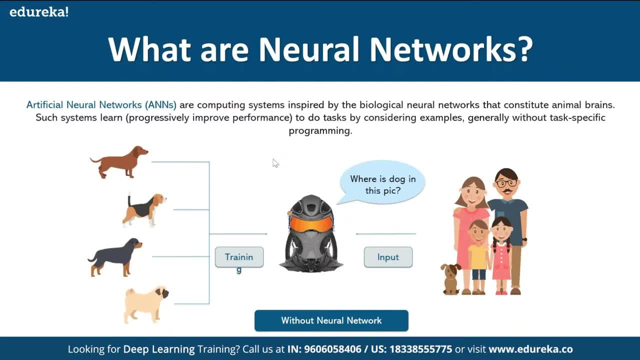 right In your mobile. your mobile can see where your faces are right. You know autofocus things are there. Similarly here. suppose you want to understand with your camera where the dog is. please locate the dog. If it is not trained for that, it will not be able to locate. But if we train this, 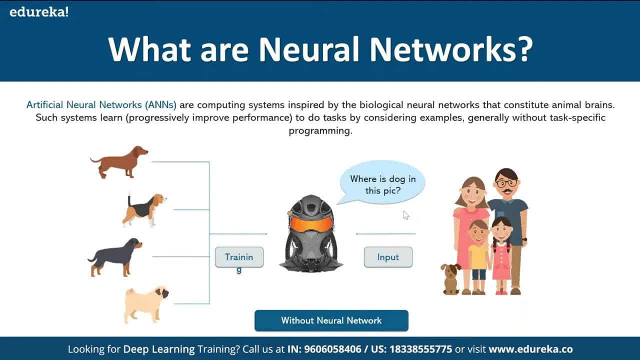 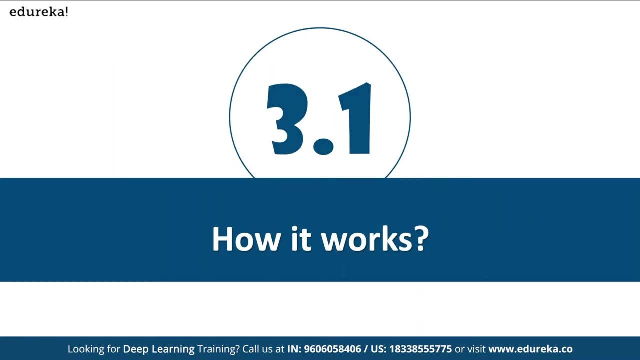 neural network with different dog images. then, after training, it will be able to say: okay, there is one dog in this pic. It will identify: okay, there is one dog in this pic, Okay. So let us try to now understand how it works. 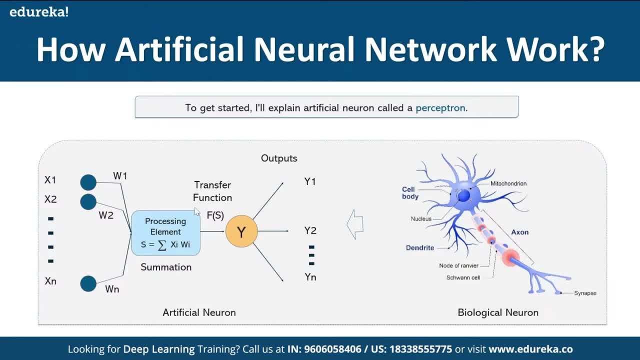 So, similar to this biological neuron, we have created now this artificial neuron. Okay, What does it consist of? It consists of three important things: One is input, which is represented by X, One is output, which is represented by Y, And there is a transfer function in between. 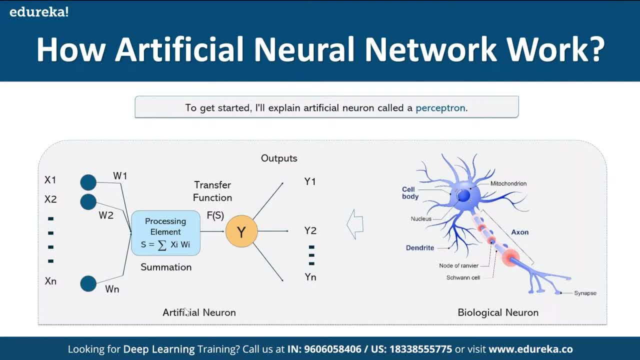 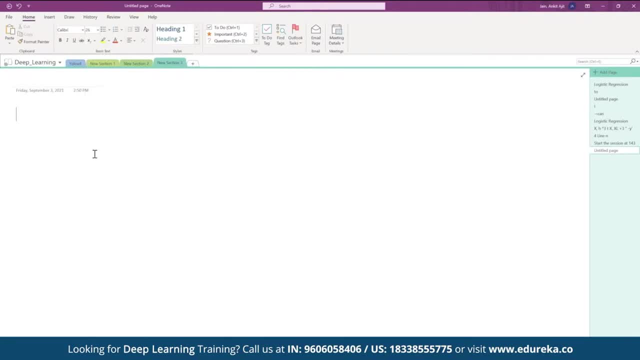 Transfer function in between. Okay, So if I have to list what are the important things you need to understand, The three things you need to understand here are input, output, weights and a transfer function. So input is represented by X, Output is represented by small y Weights are represented by small. 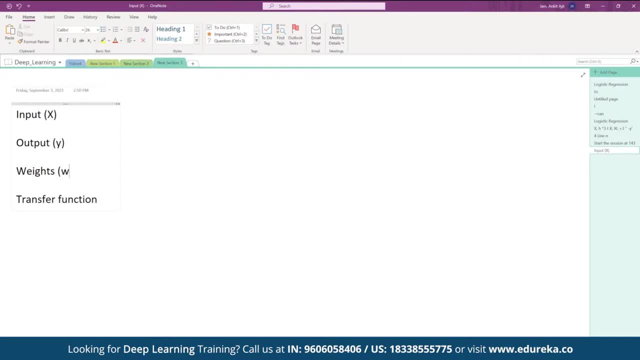 w or capital W, And transfer function is a transfer function in between. Okay, Okay, Okay, Okay, Okay is a equation which I will explain you. okay, so again, what happens is, let me give you a practical understanding. suppose this is your neuron. okay, suppose, 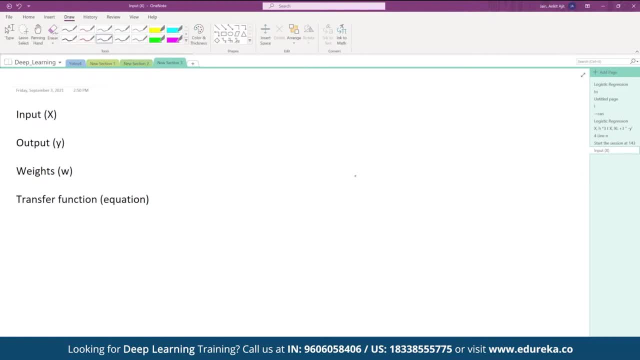 this is your neuron. suppose this is your neuron. okay, and now I am giving an input to your brain: welcome to edureka. okay, now these three words will go into your neuron right from your ear. it will go to your neuron. so what are these? welcome to edureka. these are your input: X, 1, x, 2. raise your hand, that X. welcome to edureka. 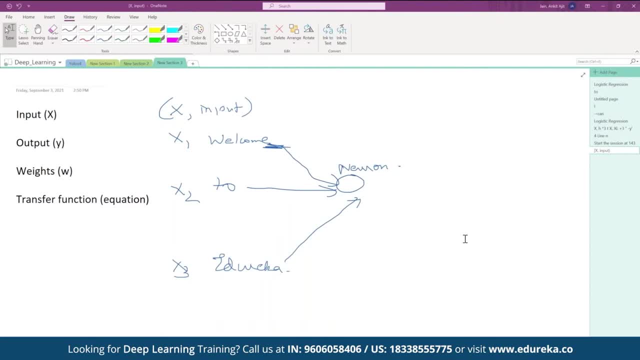 is x with an input to your brain. so, but welcome to edureka, means your input to you brain is your input to your neuron. okay, suppose, imagine this data, it is an input to your brain. okay, now, in this suppose i say uh, which are the important word here, which is the most important? 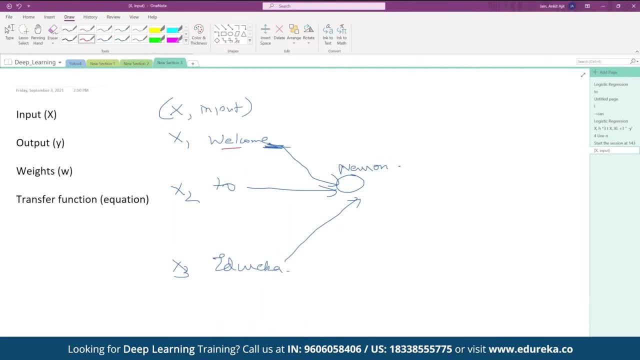 word. are all the words more important here? no, the most important word is welcome, correct. so what will be the output from this? your output will be what your output will be. you will also say thank you, correct. now. when will you say thank you? when you will listen to the word welcome, right. so most. 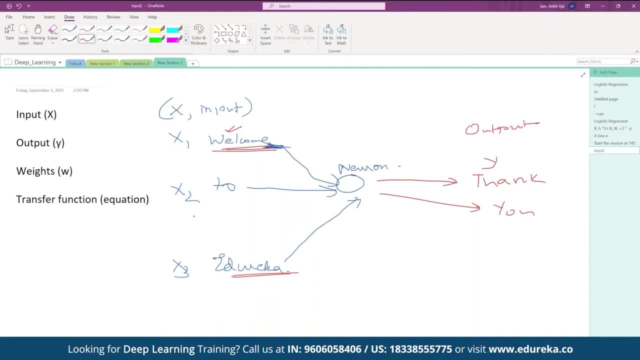 important word is welcome, and the second important word is edureka. the third least important word is two right, so all the words are not equally important here. there are some weights associated with it, so the neurons will receive this input with some weights, okay, so suppose i say this is: 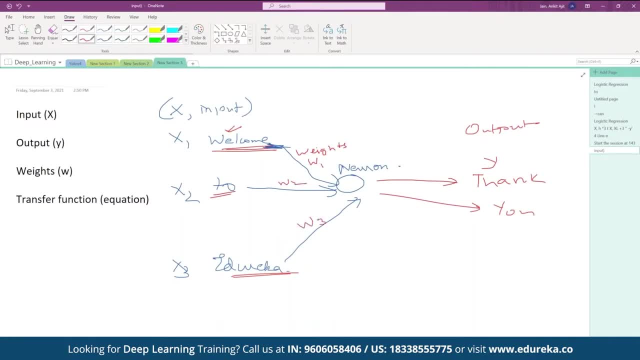 w1, this is w2, this is w3. the input is given, some weights are associated with it, right? so total total information which goes to a neuron are what it is. total information which goes to a neuron is x1, w1 plus x2, w2 plus x3, w3. okay, so these are the three inputs, three weights, total. 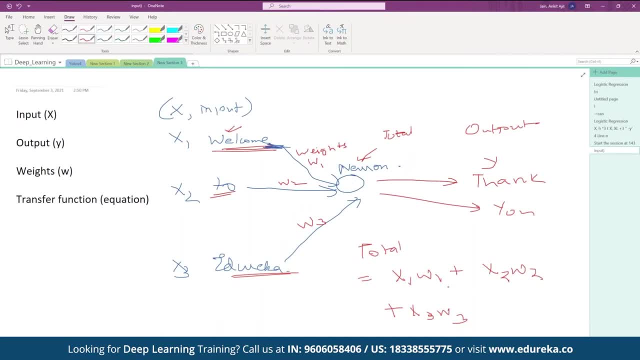 information is the product of them, plus addition of them. so this is what goes to a neuron. now, what does this neuron do? it will process this information, this total information. what it will do? it will process it. it will process the total information. okay, how will it do that, the total? 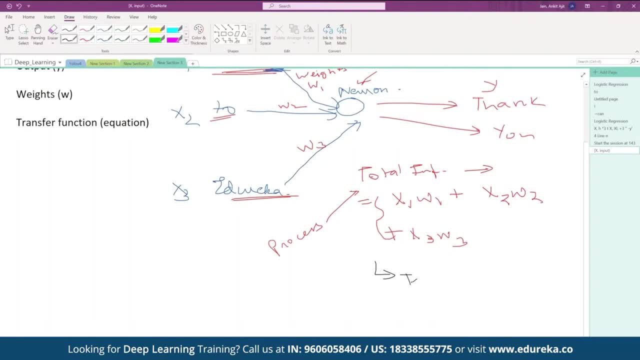 information it will process by applying a transfer function. so, just as our brain does some multi calculation, we will apply some transfer function on the total information and then we will release the output. then we will release a output. y. so x is the input. we apply weights to it. w, that is sigma. 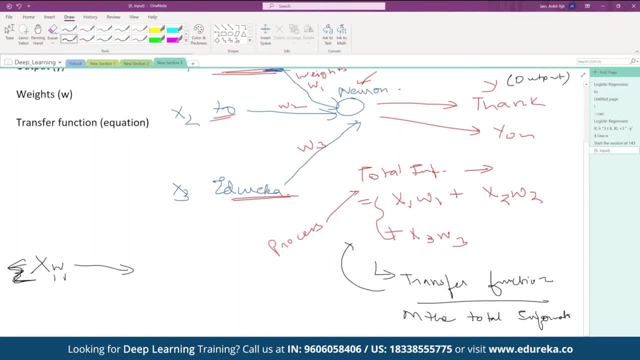 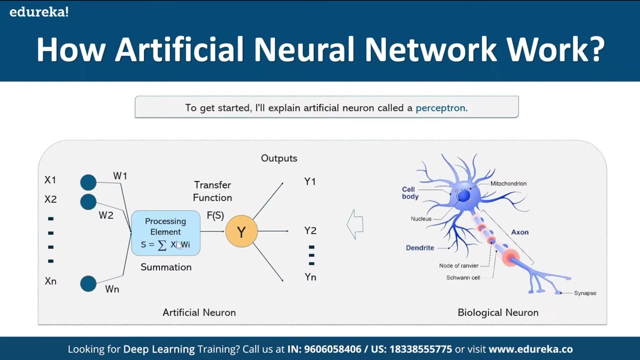 sigma xi, wi. we apply a transfer function to it and it will give you a output: okay, so this exactly is given here. we have a input, we apply w, weights, we, we do the summation of the total information, we apply a transfer function, fs, and we get a output: y. now what is? 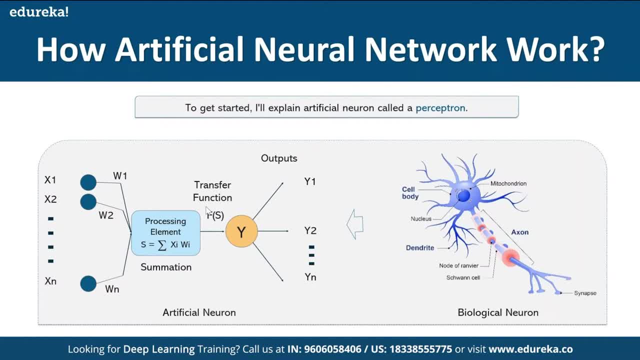 this transfer function. we will understand that. for now, just just understand that there is a transfer function applied. okay, so this is why it is called artificial neural network or artificial neuron. the reason is it mimics. it mimics the biological neuron. It mimics the biological neuron. Therefore it is known as. 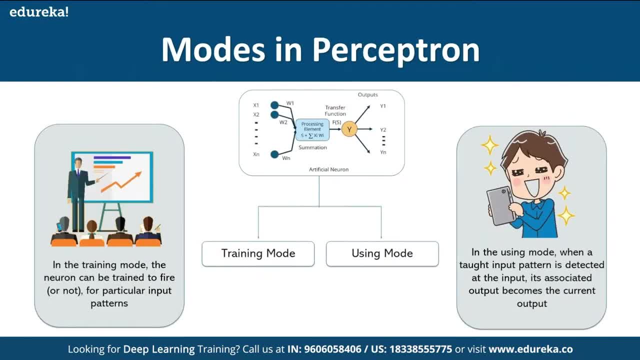 artificial neuron. Now how can you use this neuron right? So the neuron works in two modes: training mode and using mode. In the training mode, what happens is the weights are locked. We will lock the weights. and in the using mode, we will not change the weights, We will use the. 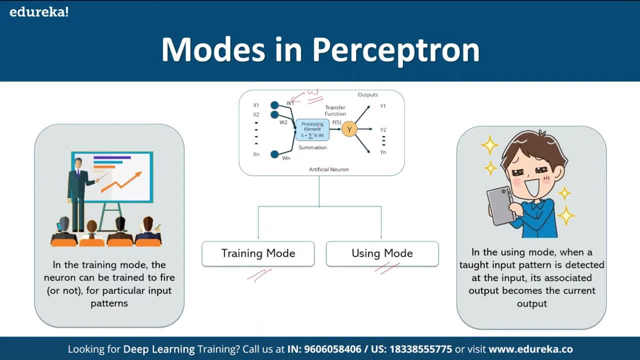 neuron as it is To make it more interactive for you. to make it more interactive for you, it is something like this: Once you recognize that, suppose my name is Ankit, right? Suppose you recognize that this voice today you heard it for the first time. right, It represents Ankit. 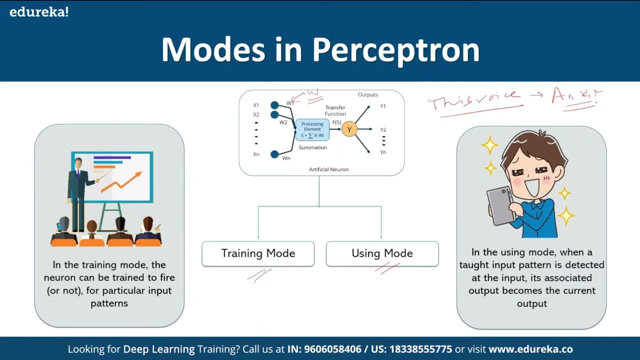 Now your mind knows that. okay, the voice I am listening to is Ankit. Now that is your training mode. You are being trained, right. So one hour you will listen to me. You are getting trained today. The next time, if I come and speak to you, right, you will not be required to train Your weights. 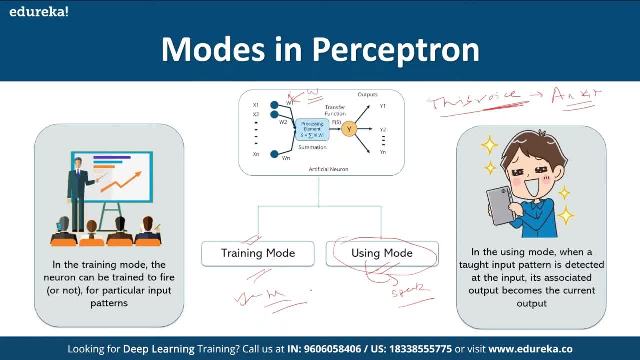 will be locked. Why? Because you have already been trained with my voice. Now, next time when I come, I don't need to introduce myself. As soon as you listen to my voice, you will say it is Ankit speaking. right. This is how we identify most of the actors, right? 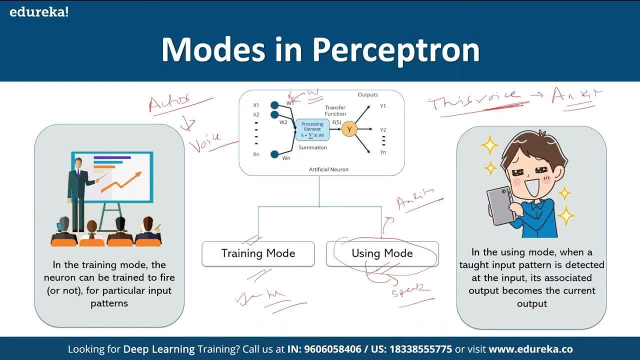 We understand who it is by their voice, also because we have been trained to listen to them, right. Similarly, our parents are all know, right, They are trained. So when we see modulation in our voices- right, they understand what emotions you are going through, right. Are you tensed? 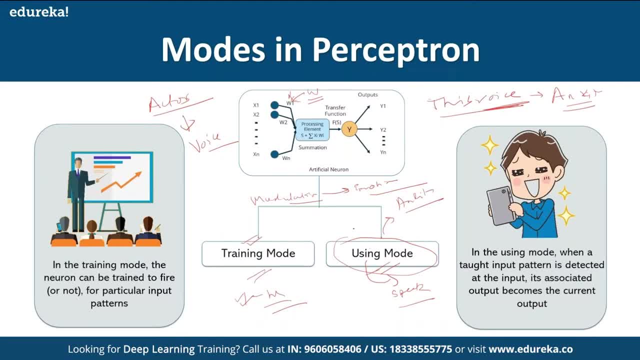 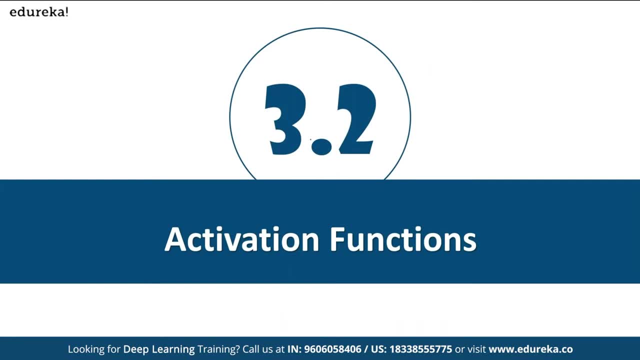 Are you feeling worried? Are you happy? right, So that is the training mode and the other is using mode. okay, Now, what are transfer functions? We will come to that. Okay, So transfer functions are also known as activation functions. Is it clear? Transfer? 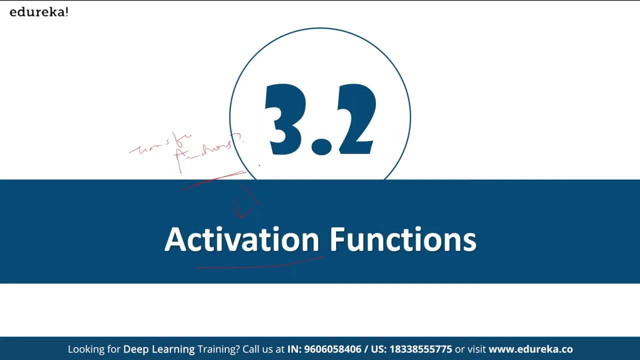 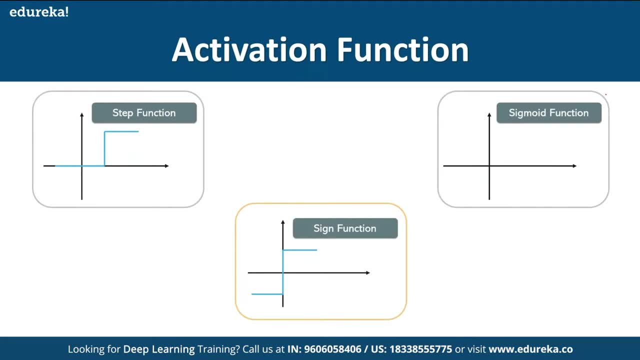 functions are also known as activation functions. Now, what kind of transfer function we apply? We basically apply a match part to it. We may apply a step function. So whatever information you are getting, always remember we apply activation function on the total information. So, whatever. 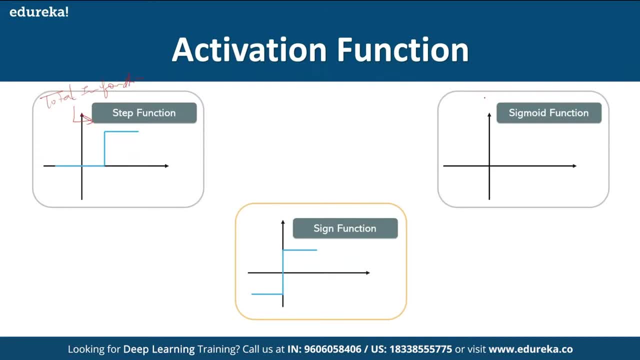 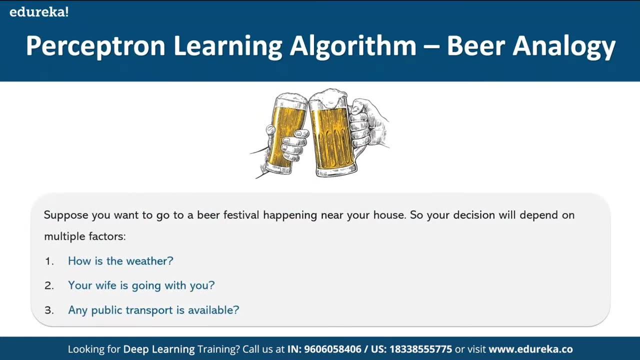 information you are receiving, you will apply either a step function, a sigmoid function or a sign function or some other functions. So basically, your information comes and you have a function applied to it. I will give you some practical understanding. So let us first try to understand this. Suppose you want to go to a beer festival. 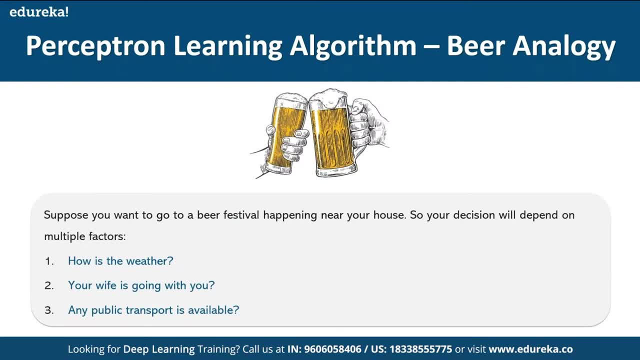 happening near your house. What will be your decision, depending on whether you will go there or not? It depends on how the weather is right. If you are going to a beer festival, you may want to go to a beer festival so that you can consume your beer. you can enjoy your beer right. But if 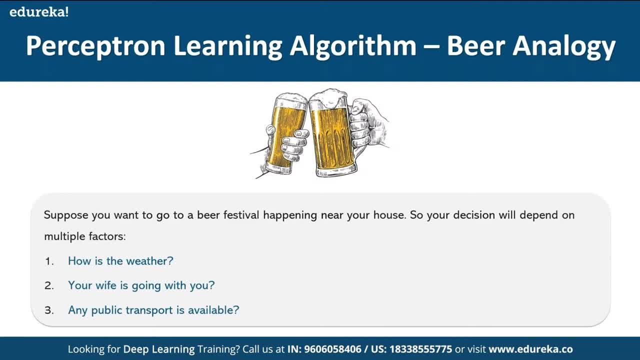 the weathers are not conducive, you will not go. So first is weather. Second is who is accompanying you. Is your wife going with you? Is your friends going with you? So that is another important factor. And third is what transport you can use to go to the beer function. right, So can you go. 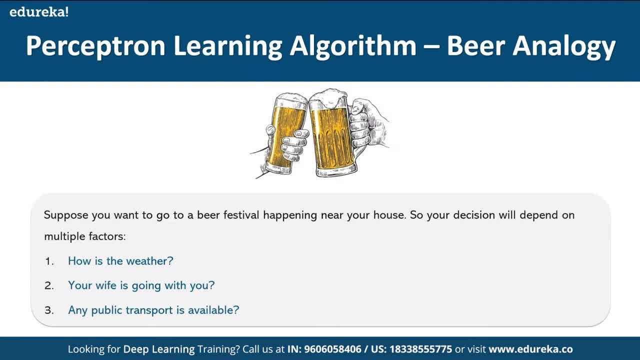 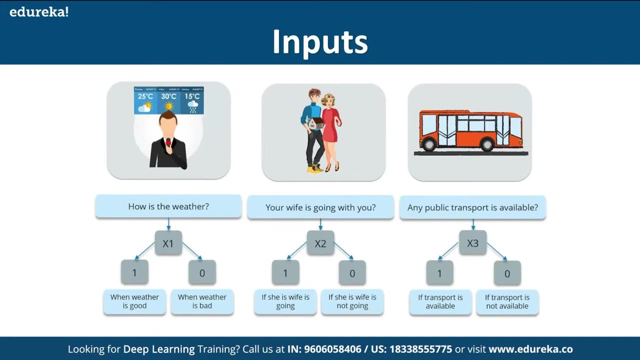 by car or you will take a public transport right. So, based on multiple factors, you will take a whether you should go to the beer festival or not, right? so let us first try to understand each of the parameter so your mind will understand. how is the weather? x1, so the first input is x1. 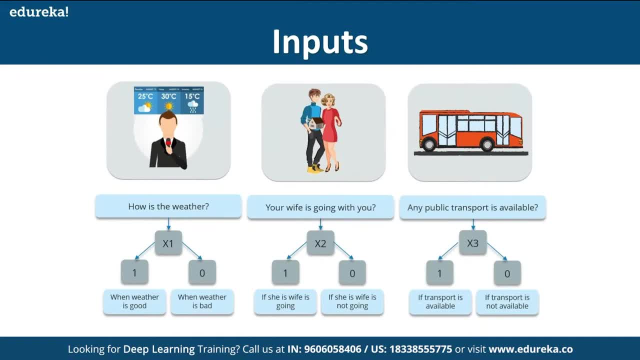 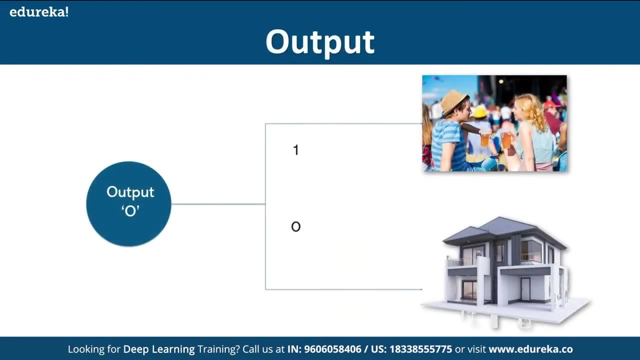 if it is 1, it indicates whether is good. if it is 0, it indicates whether is bad. your wife is going with you. x2 is your second input. is it yes or no? public transport is available? yes or no? that is your third input. and what is your output? yes, you may go to the beer festival, or zero, you may not. 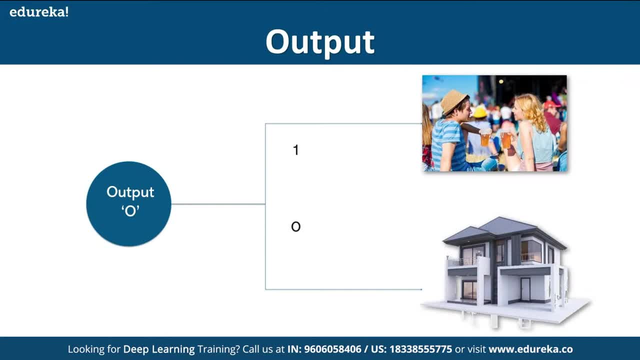 go to the beer festival, you may remain at your home right. so the possibilities are clear for everyone. input are x1, x2, x3. three inputs are possible: x1, x2, x3. three inputs are possible, and in every input you have either 0 or 1 right, and output is also 0 or 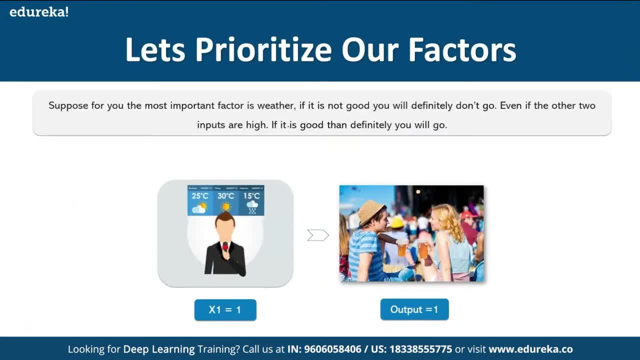 1, that is represented by y. now let's prioritize our factors. so the first factor is: the weather should be good. x, 1 is equal to 1. then for sure your output is 1. right, if weather is not good, obviously you will never go, but if the weather is good you will go. then we will assign the weights. 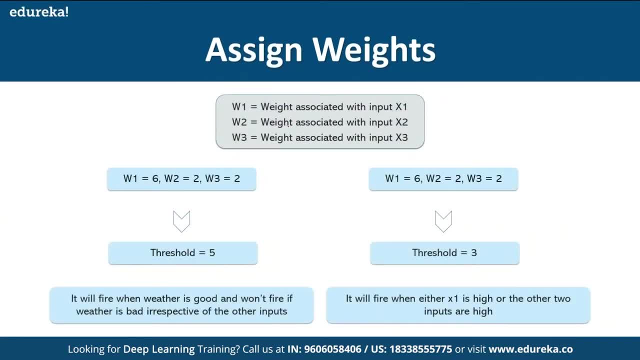 so, according to each factor, we will assign the weights. for example, weight associated with x1, weight associated with x2, weights associated with x3. so these three weights, say example 623 or 622, it will give you total information value and, depending on total information, if it say: if it. 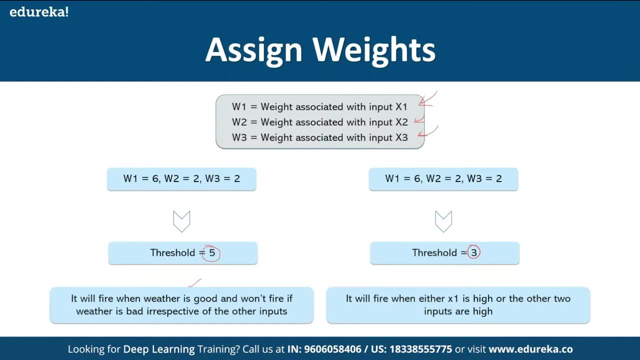 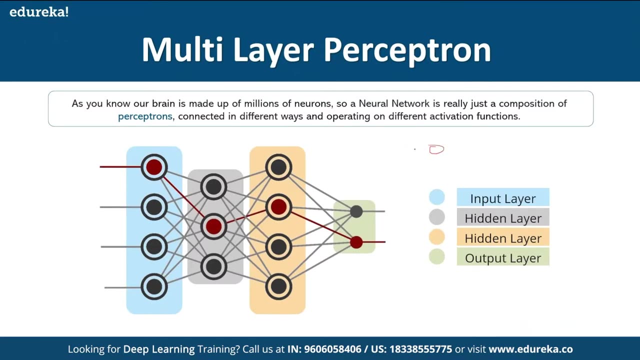 is greater than 5, then you will go. if it is less than 5, you will not go. so there is a threshold. that how much is the threshold reached when you apply weight to your information? now, as i said, one neuron will consist of these things. what input right you have? 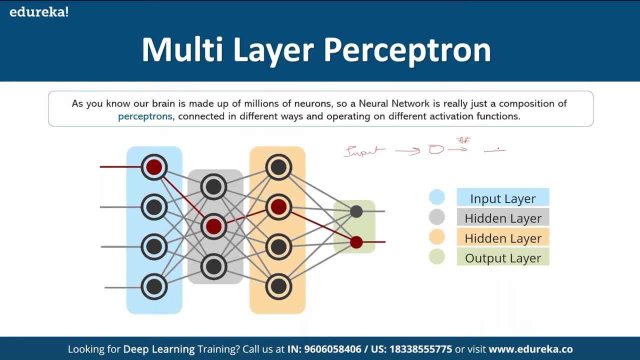 transfer function or activation function applied to it and then you get an output right. so this is what happens in a single neuron. now, each neuron is connected to each other. so if you see a human brain right, you can see four neurons are connected to three neurons. 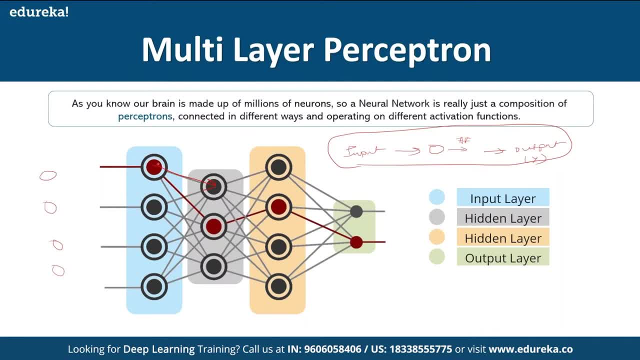 Now it is not like this neuron will only be connected with this neuron. No, it will be connected with other neurons also. So can you all imagine now the complexity of your brain. Every neuron has weights. So if you see here 1w1, w2, w3, w4, input weights- 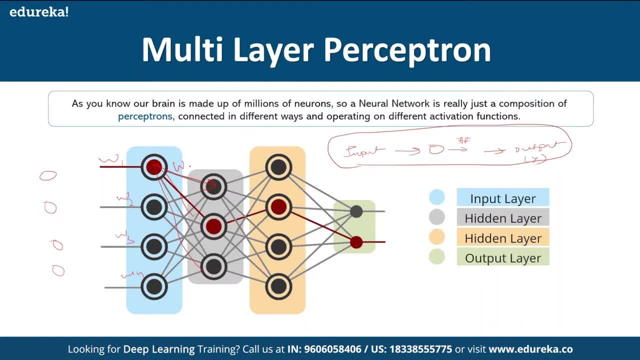 Similarly, in your mid-layer you will have weights associated with each neuron: w11, w12, right, it is also going to w13.. So total nine connections will be here, right, and then each three is connected to four other neurons. So these neurons in between are 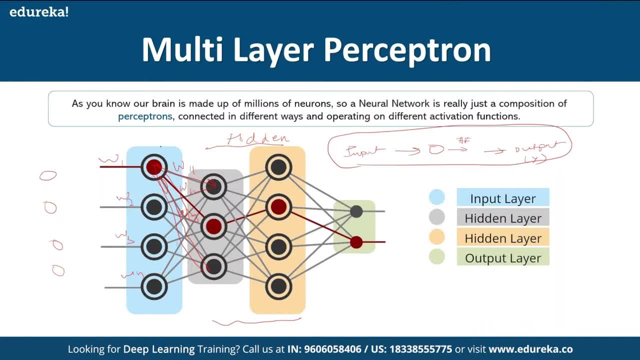 known as hidden layers. This neuron is known as input layer And this is known as output layer. Can you all imagine now- It is your human brain- where each neuron, every neuron, is connected to each other. Okay, So which is the hidden? 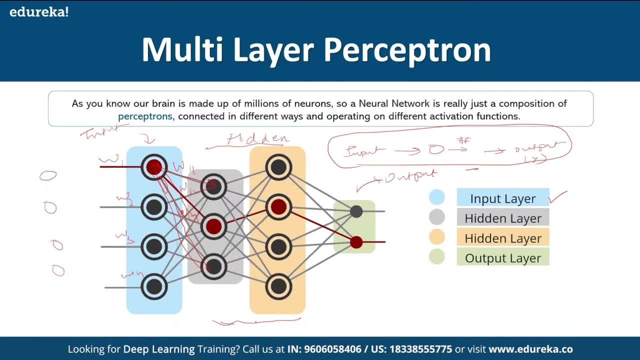 which is the input layer, the blue one you can see here. these are your hidden layers and this is your output layer. Now I can explain you the term deep learning. You may have heard about it, Right, deep learning. So deep learning is nothing. 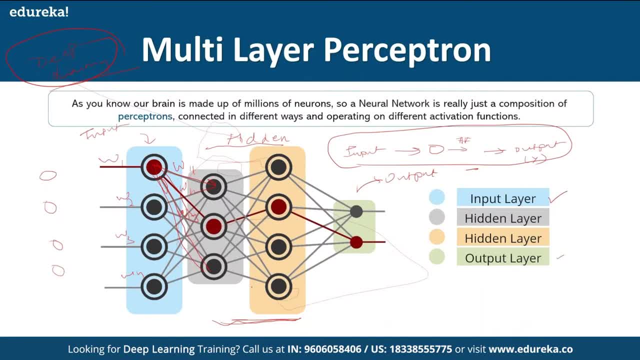 a neural network in which your hidden layers. a deep learning is nothing, but your neural network is greater than one. so if your neural, if your hidden layers are greater than one, we call it deep learning. i hope you are able to associate yourself now. the deep part is because you are. 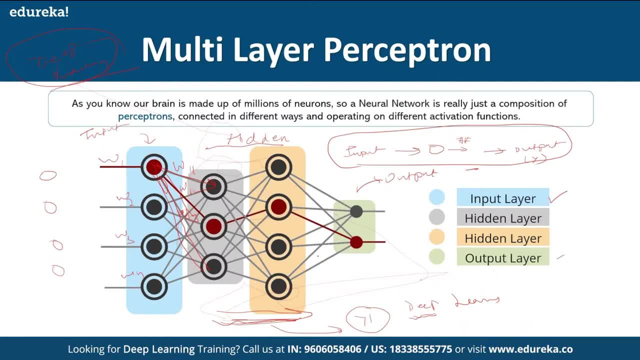 learning, trying to learn deeper. you are having more layers between input and output. you are giving more thought to your process, more process to your thought. and second is you are learning through this artificial neural network. that's why it is known as deep learning. okay, the hidden layers where we apply the function and the number of neurons. 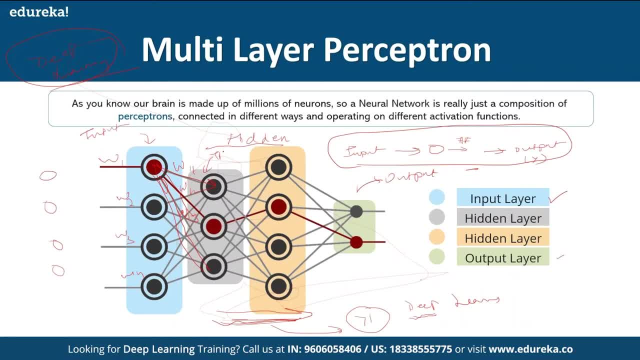 yes, in the hidden layers also we apply transfer functions. so every neuron, you will see there is transfer function after it and there can be more neurons. you can have hundreds of neurons in a single layer and there can be multiple hidden layers. you can have two, three, five, ten, whatever. 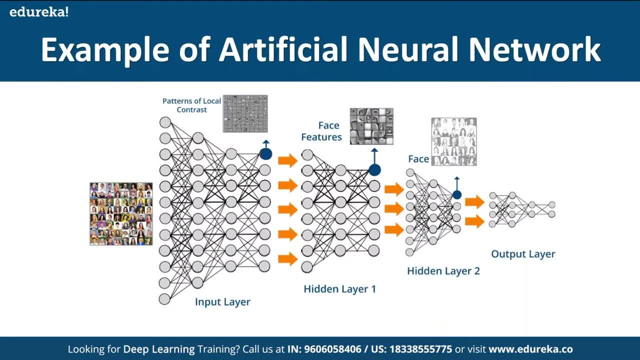 you want. so this you will see examples. suppose you want to process each of the faces on this image. okay, what you will do. you will pass it through various input layers, you will pass it through hidden layers and then you will get an output layer. so here it is, showing that after, after, 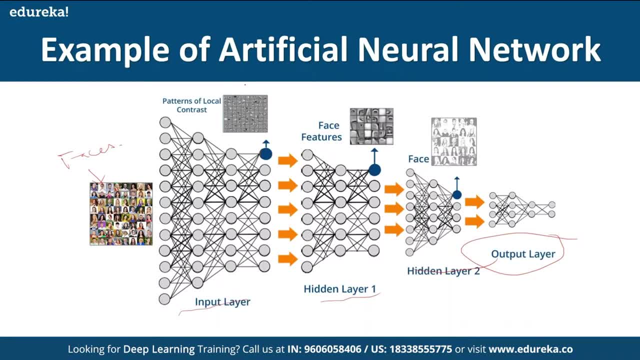 doing some, you know, manipulation over this data. this is how this image will look. this is how it will look at the end, after the output, you will be able to see, okay, each image. you will be able to identify who is there in that image. okay, so such kind of complex neural networks we have to. 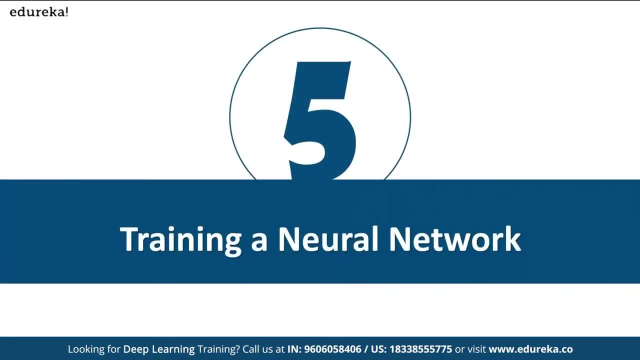 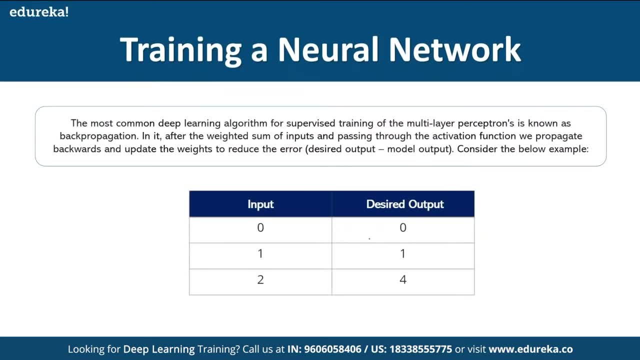 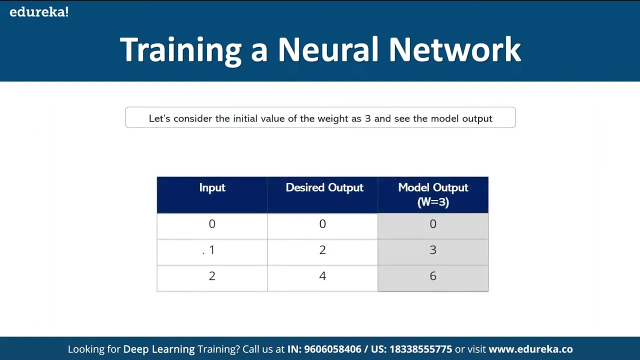 develop. now, how do we train a neural network? so we train the neural network. for this, there is a concept known as supervising learning. what is it known as supervised learning? now, in supervised learning, what happens? you have an input and you have an output, so there is an input layer and there is an output layer. and what will your model do? 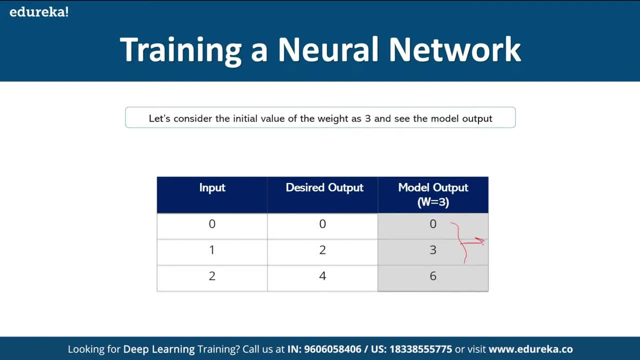 your model will assign the weights to it. so this happens. this is your model output. so you have your input and you have your output. in between, say, you have one hidden layer. now every neuron is connected to other neuron and there is a weight associated with it. who will? 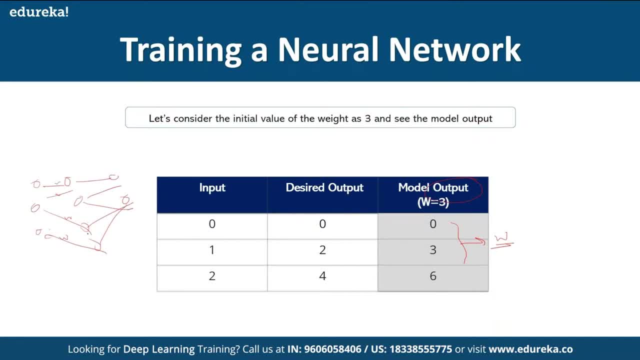 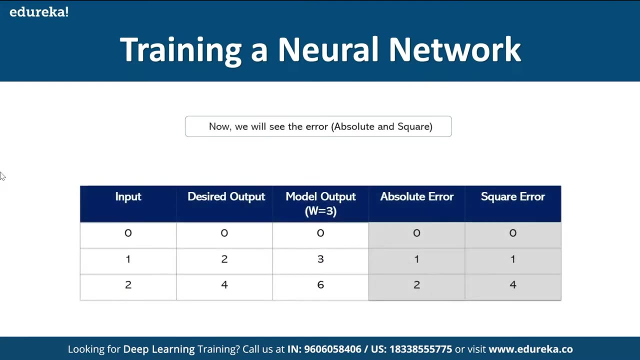 assign this weight. this weights will be assigned after you do training of this. after your training has been done, these weights will be associated, identified by a model that will be your model output. okay, so what happens initially? you have an input, you want output of zero and you have a model output of. 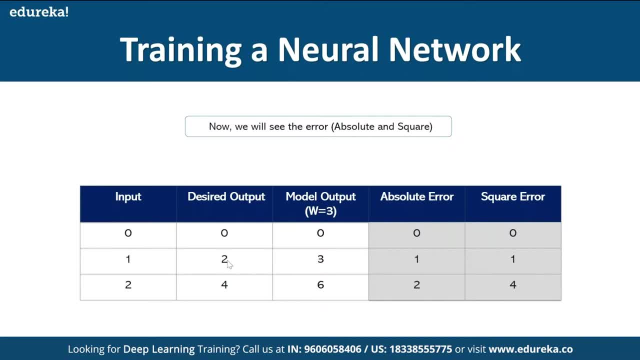 zero. here your input was one, desired output is two. but what did your model give? your model gave three. here it was two, your model output is four. so if you see, your input and output are double of each other. but here, what your, what your model or neural network is giving, you are giving an input. it is 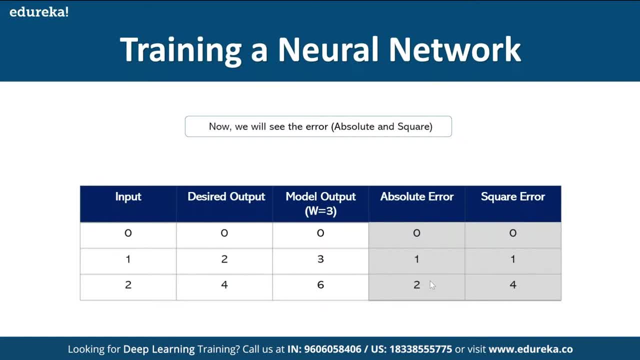 returning value of three. so there is a value of three. so you have a model output of zero and you you have a model output of zero, but here your model and input are two, so you know the value of three. there is an input error in there saying error of four, and there is a difference of one right error. 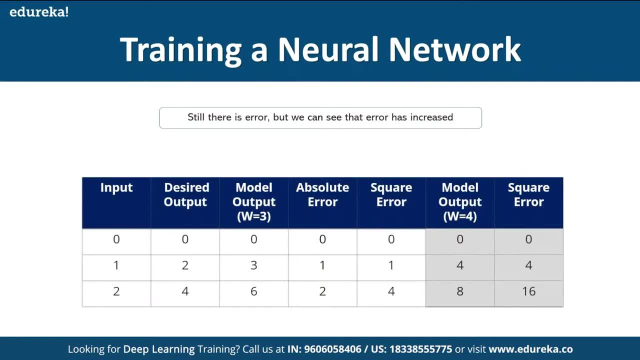 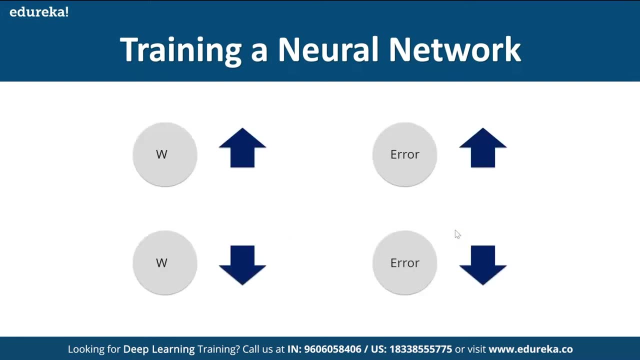 of one error of two. so what it will try to do is, basically, it will try to minimize this error. okay, it will try to minimize this error by adjusting the weights. so if you see as and when it adjusts the weights, you start. so suppose you now keep a weight of 4 instead of 3. this is the values you are. 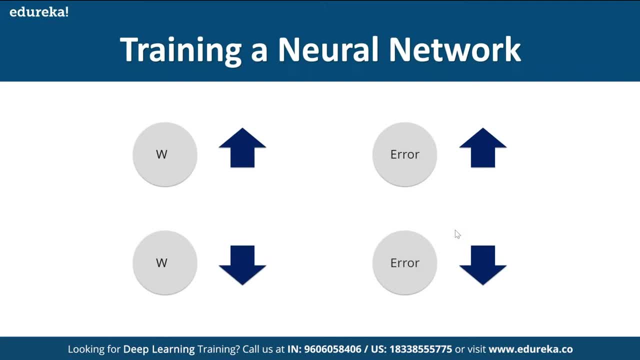 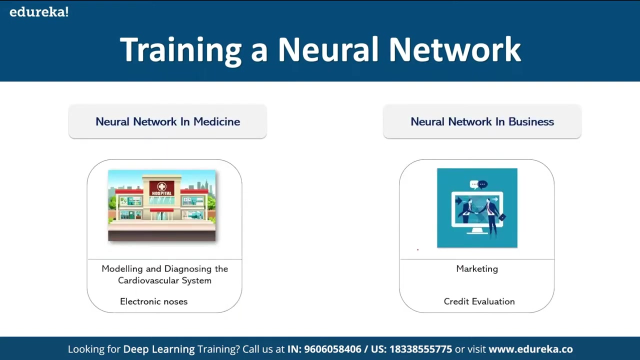 getting right so that your error can reduce. So if you see, at one point of time, the weights right, at one point of time, the weight at particular weight value, your errors are zero. your errors are zero. this is the weight of your neurons which will be locked. So where are the neurons used? 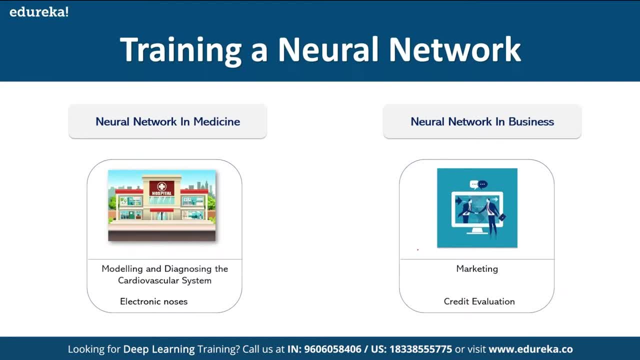 neural network use. the neural networks are used in medicine, in business, it is used everywhere. okay, so your Alexa, okay, all your- you know- face recognition technologies, all of them are using neural network based models. okay, so suppose you give a x-ray. okay, suppose you give a CT scan. 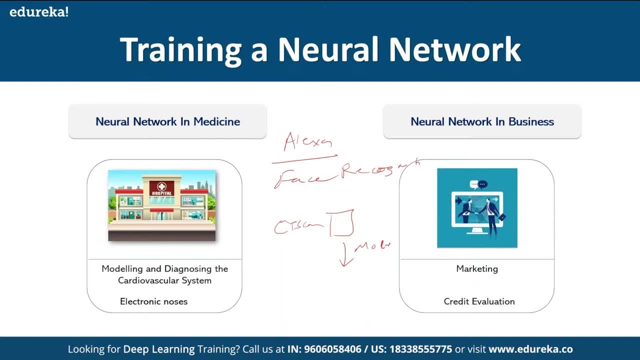 and your model will detect whether it is a covid or not. okay, so this model usually are artificial neural networks, so it is used in a lot there: electronic noses, now you have, you know, sensors which can sense the smell, which can sense the smell for use it: a good smell, bad smell in hospitals, and all so those. 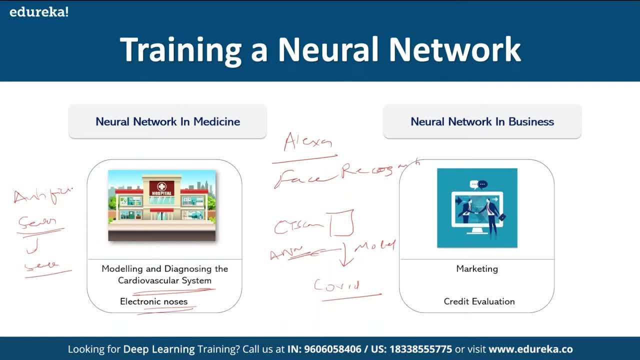 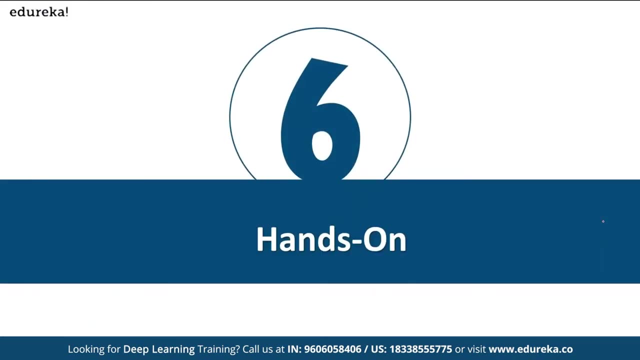 sensors, artificial sensors are also using artificial neural networks. Similarly, in business, for marketing, for credit evaluation, whether you should give that person the loan or not- all these things you will get using neural networks. So let us do a hands-on session now, let us try to create a neural network. so what we will do for that, for hands-on session, we will use. 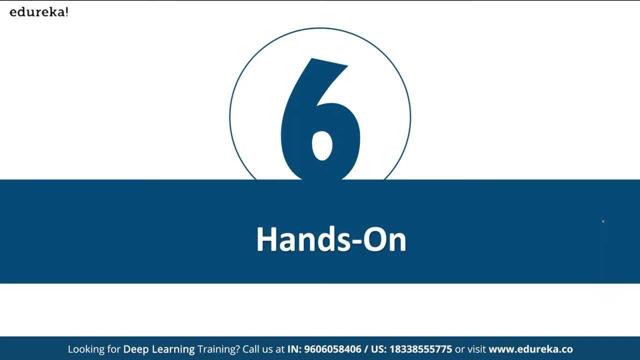 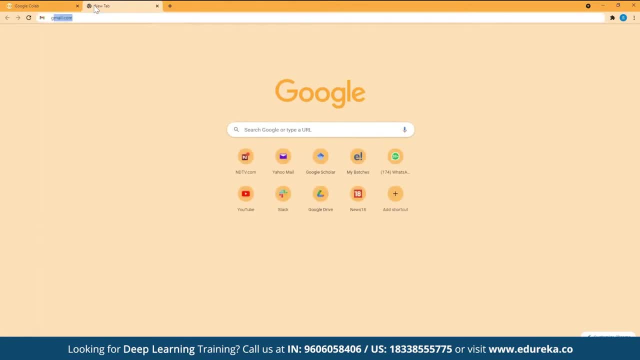 a platform. okay, we will use a platform known as Colab. all of you, you can open Google Colab. So, if you search online Google Colab, if you have a gmail id, okay, you can open this Google Colab. okay, now in this Colab, what happens is you can create a notebook. okay, you can create a notebook. 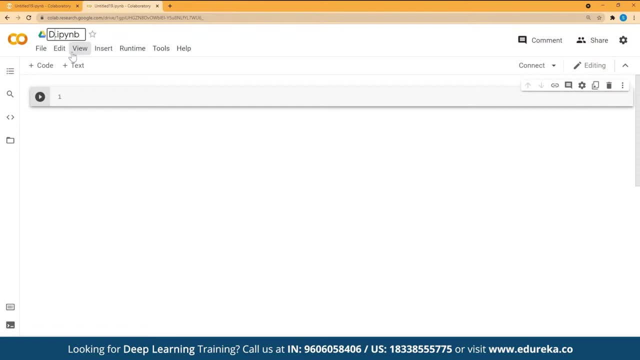 and in this notebook it is like a laptop itself. okay, so online on cloud, Google has provided you a laptop, a virtual laptop, which you can use for coding, so it has installed python for you. it has installed all the requirements for uh you know, uh doing, uh, python, coding, etc. everything has been provided to you. 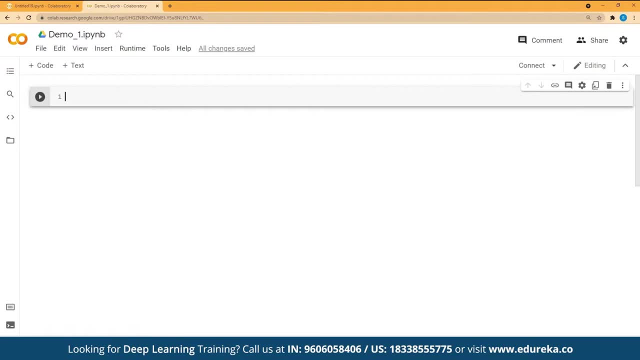 here. okay, so here, what we are going to do now is we are going to create a artificial neural network. okay, we are going to create a artificial neural network which will detect whether in the image is there. okay, for example, i want to create a neural network. what it will do is: you will train. 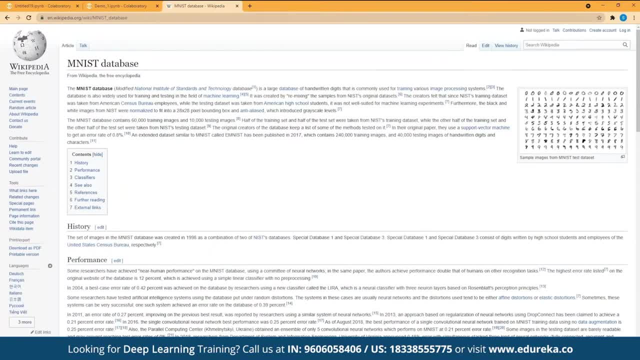 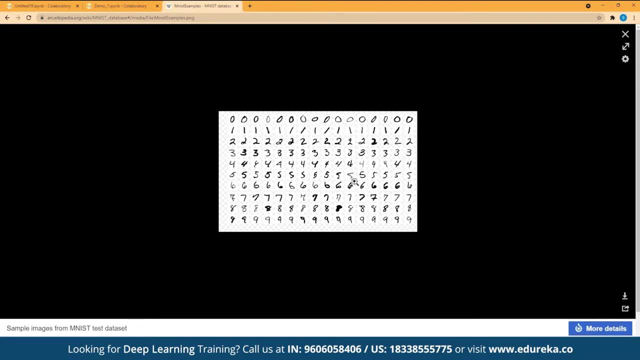 the neural network with images. so, for example, these are the images. okay, and i will train a neural network which which will read these images and it will show you that on a particular image, it is 0, 1, 2, 3, 4, so it is handwritten. but it will also understand that what number is written on the 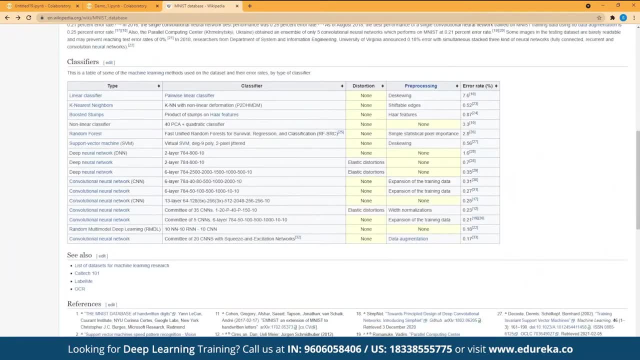 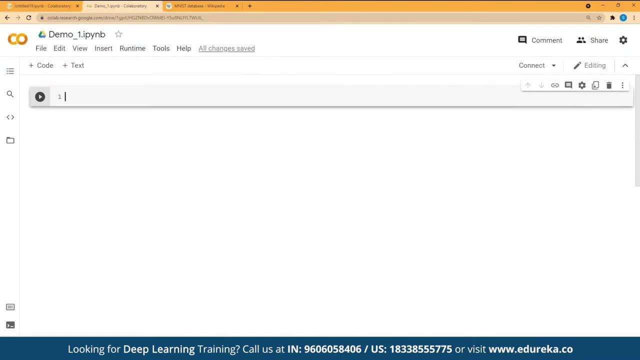 image, okay. so for, in order to train that model, we already have a mnist data set which we will be using here. okay, we will be using the mnist data set. okay, so first, what we need to do: we need to import quite a bit of models in quite a bit of packages, okay, so i'm just going to give you. 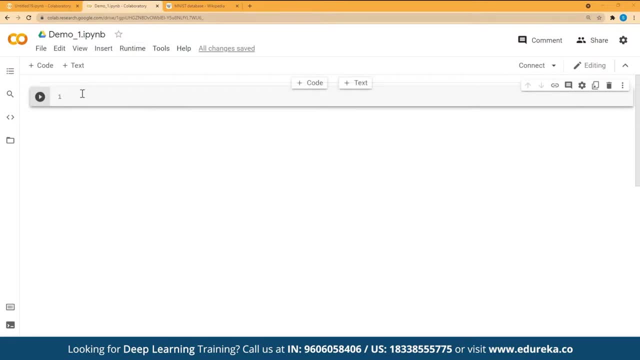 what packages we are going to use here. so we are going to use for coding, which you will learn in detail if you go for the course or you do some structured course. you will learn a package known as keras. what keras does is it uses something known as tensorflow in order to create your neural network. i will explain you. 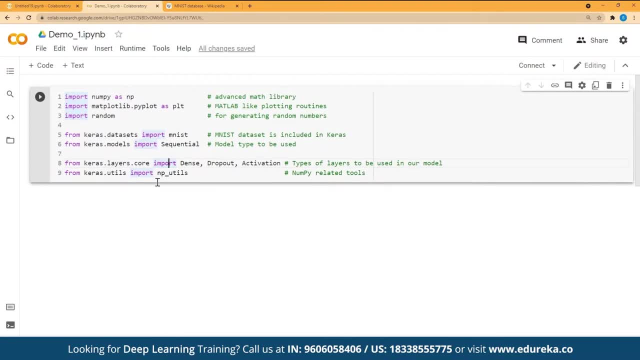 with the demo it may get somewhat clearer to you. so we are going to import all these packages. so these packages have pre-built-in uh, you know, we can create neural networks using these packages. you know, in our existing toolbox we don't need to, you know, do uh write all the algorithms it. 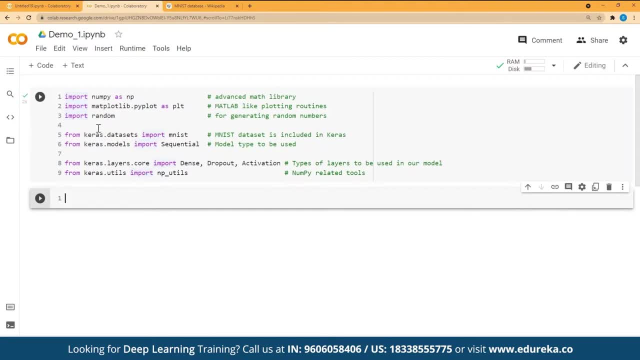 is pre-built, and what is the advantage of using collab here? all these in have been installed inside collab, so we are going to use a package known as keras in order to create a deep learning model. okay, so first, what i will do, i will load the data set. the data set i'm going to load is: 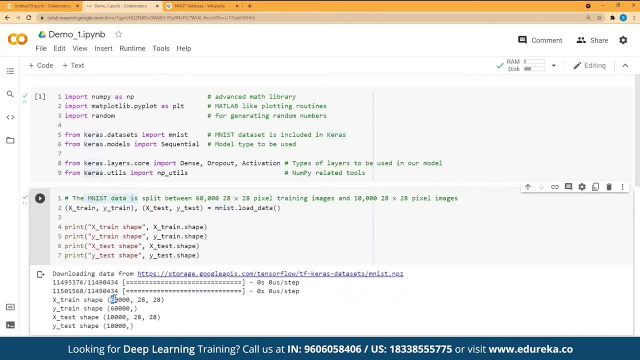 the mnisd data set. as i explained, mnisd what it contains: 60,000 images, okay, whose size is 28 x 28,. these images we are going to train on an artificial neural network and it will predict what is the number on that image. So first we are. 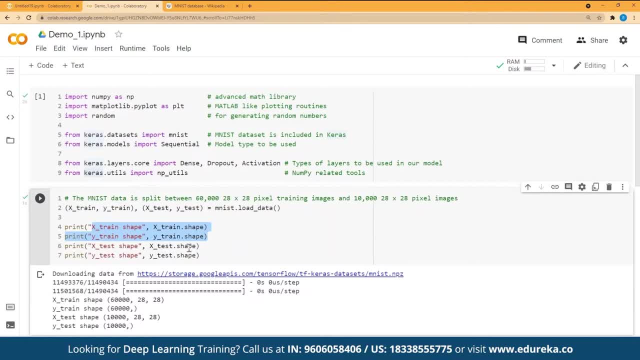 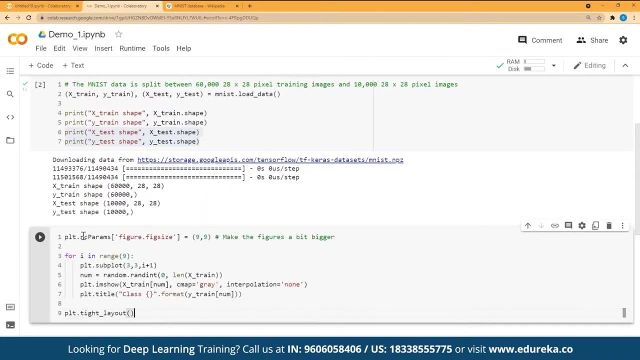 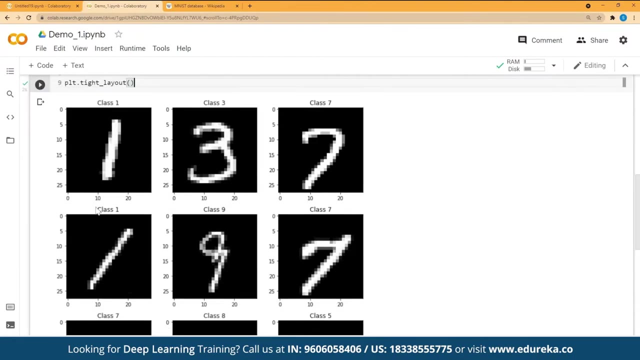 going to train that image and once that image, once that neural network has been trained, we are going to test it. Okay, So just to give you an example, how. what are the training images? these are the training images. So here, if you see there are various, this is: 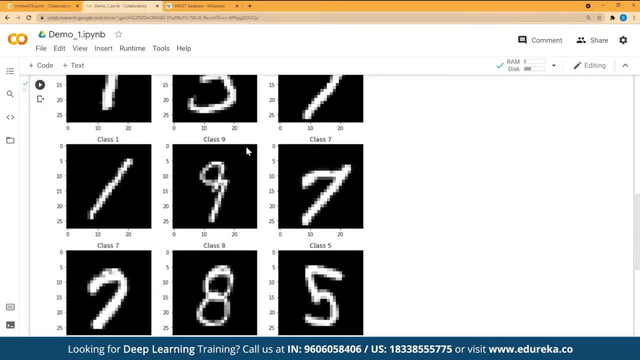 1,. this is 3,, this is 7, right, So these images we are going to send in an artificial neural network, as I just explained to you, and that weights will get locked and later, when we send an unknown image to it, it will identify. okay, this number represents 3.. 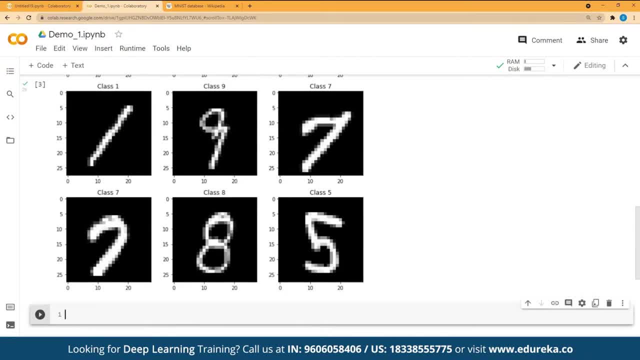 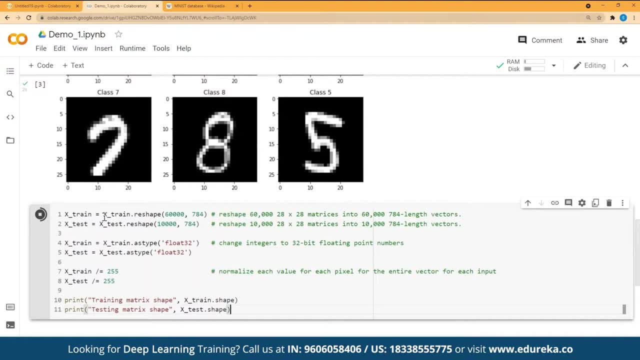 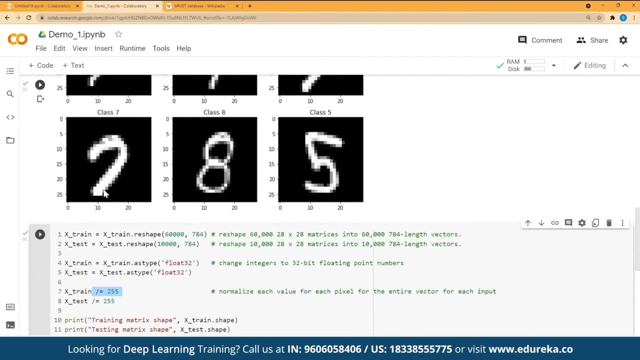 Okay, So this is the practical aspect of this hands-on session. Okay, So I will do some data processing First of all. what I will do? I will try to scale the data here. So see, you also have to learn a few more concepts here: What is the image, What is a pixel, etc. So if you 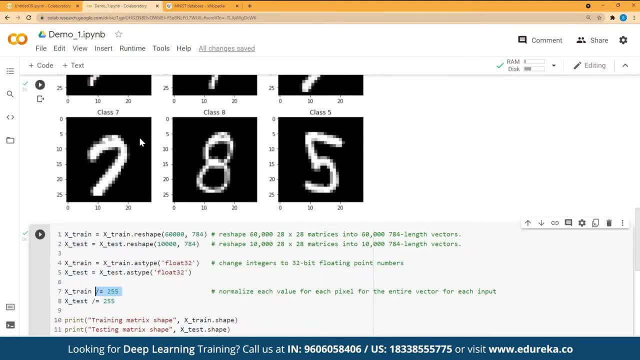 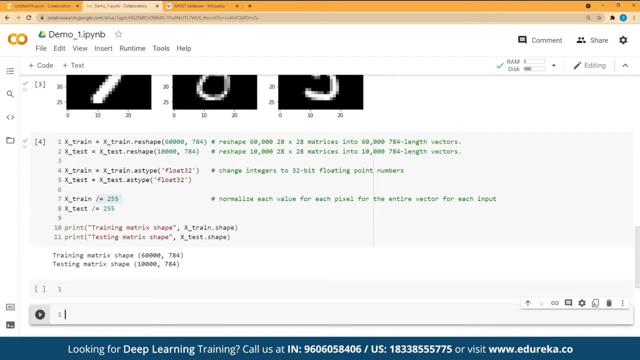 know about that. what we are doing is dividing this by 255, now, 255 is the biggest pixel we can have in this. Okay, So we are normalizing all the pixel values on these images by dividing it by 255.. 55. Okay, Now, what I'm going to train is this. What I'm going to create now is this data: 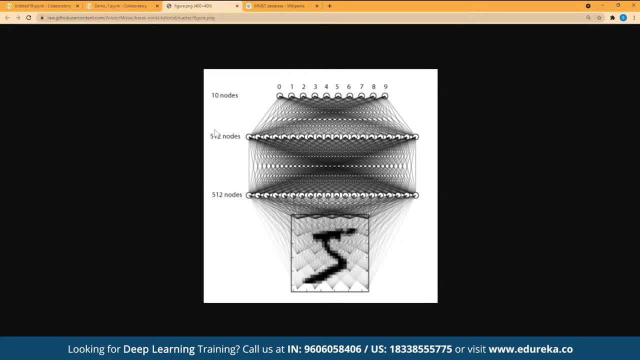 So I'm going to create hidden layers of 512 nodes, So 512 neurons. The image will go as an input to these two layers of 512 nodes and it will give you output of 10 variables, So it will give you the probability of what is there on this image. Okay, So first of 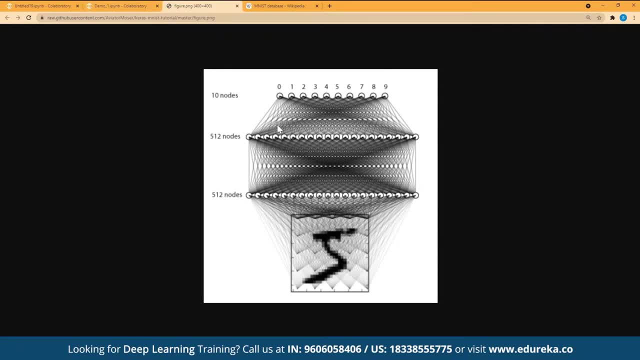 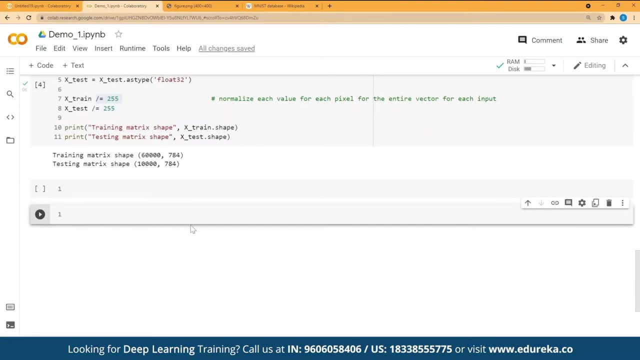 all, we will train this and then we will use this neural network in order to get it, in order to use it. So first we are going to train it, For that I will have to create a model. So I'm creating a model. Model equal to sequential. So this is the code used to 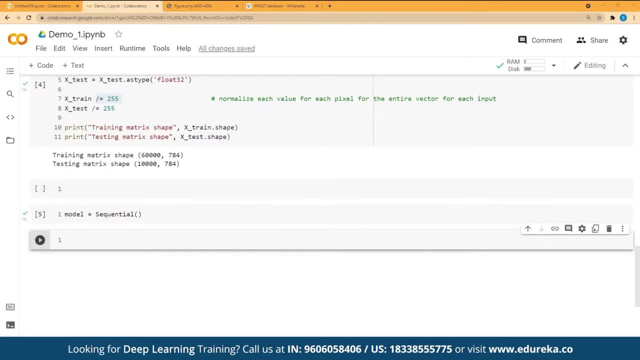 create a neural network. Now you will see with the ease with which we will create the image, The neural network. Okay, So I just need to say, please add a dense neural network. We also call this dense neural network, the image I show you. So I'm telling you: please, 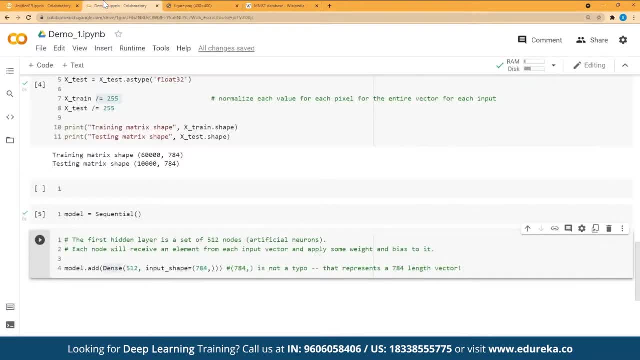 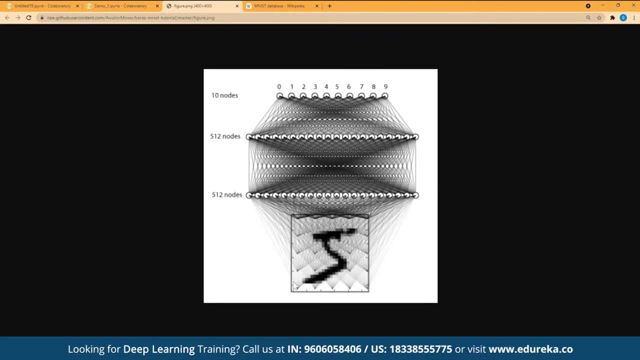 add one layer of 512 neurons. So it is doing that 512 neurons. What will be the input to it? 784.. Now, 784 are the number of pixel values in this image 5.. So we are telling: please me, to add one layer of 512 neurons. So here is the input into 512 nodes. Okay, So this? 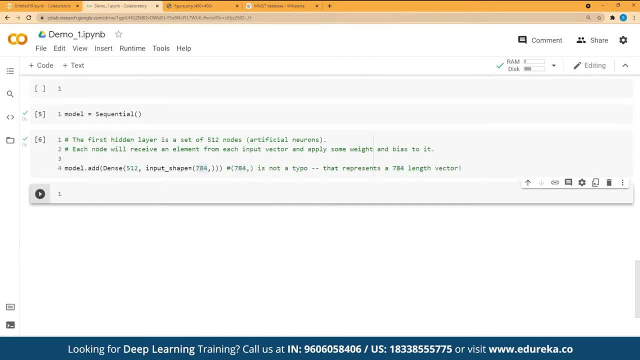 is my first layer, First hidden layer. Then what I will do? I will add an activation function. You remember I explained you activation function. So we are going to use an activation function, known as ReLU, here. So after it goes into the dense node, we apply activation function. 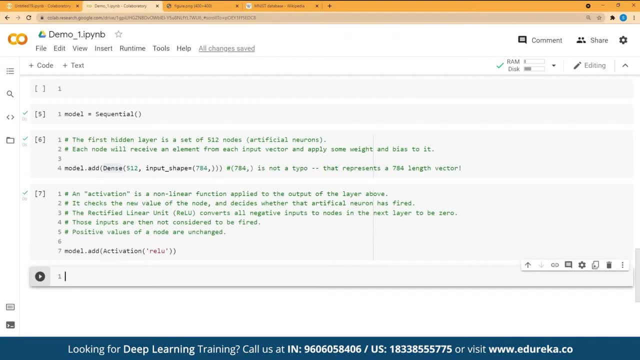 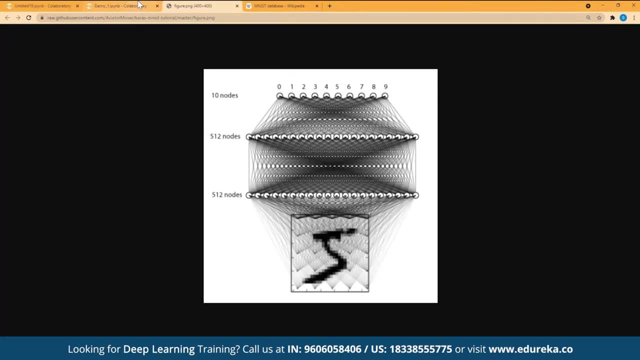 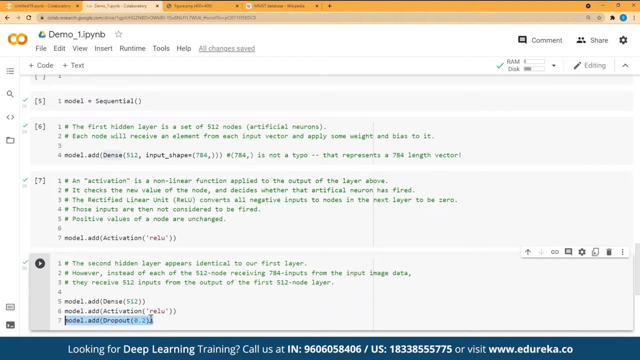 Then again what? we will have another dense node, We will add another dense node, Then we will add another activation function, then an output. so this is how we will do that. okay, now there are some concepts of dropout etc. i will not go into those details, but those are. 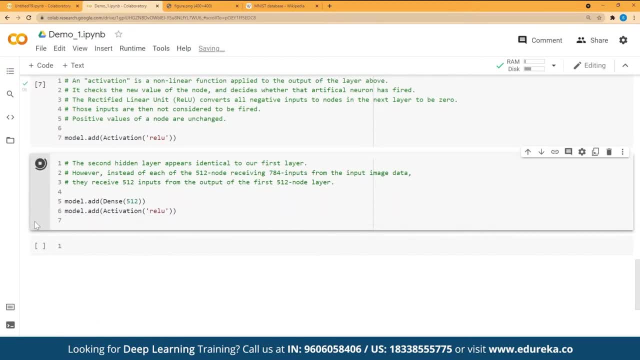 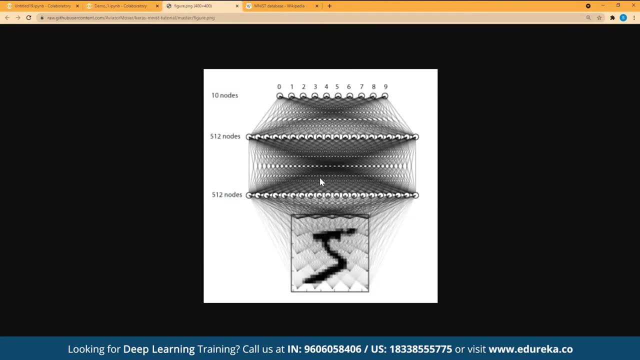 higher concepts. here i may remove these dropout players also. so for now, what i have done, i have, if you can understand. i have created the first layer, i have applied the relu function over it. now, whatever output is going, it will go to the next layer of 512 nodes. you can check here. 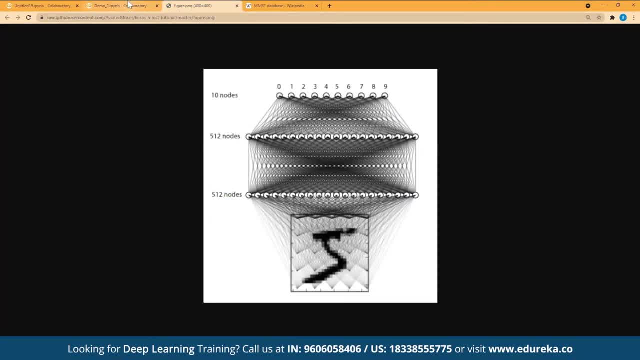 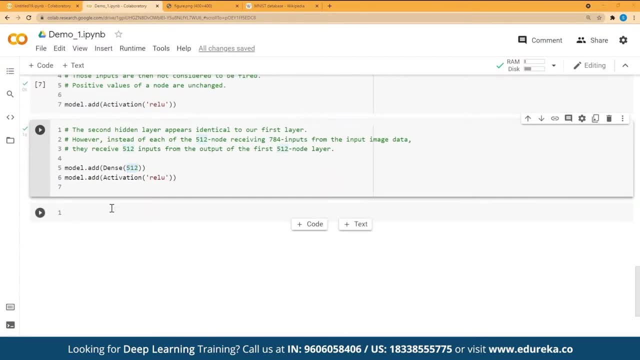 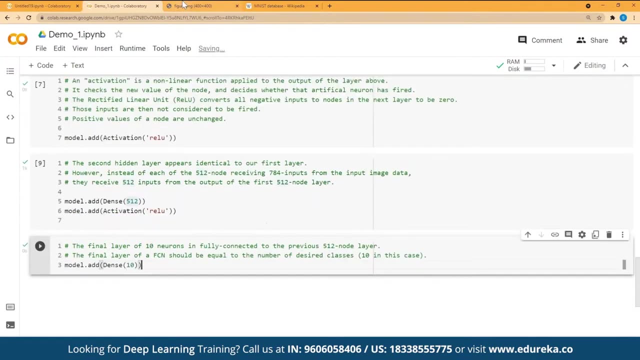 next layer of 512 nodes, and then we will have a output layer. so now i will create the output layer. how i will create it? i will just write model dot, add dot, dense 10.. so now, with this four, five lines of code, you have created this complex neural network. okay, you have created this complex. 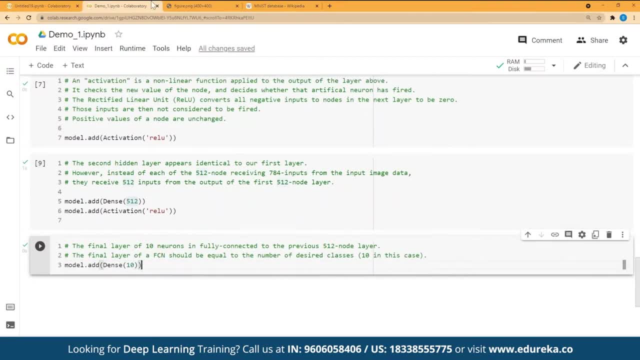 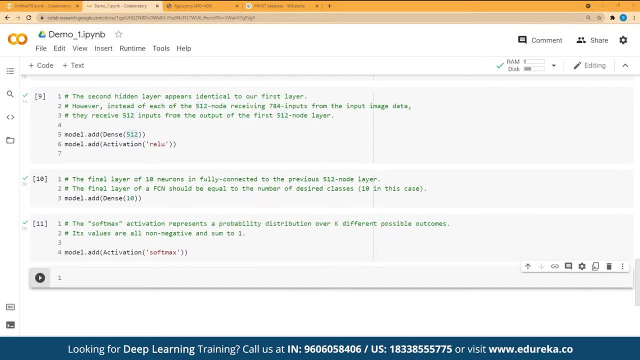 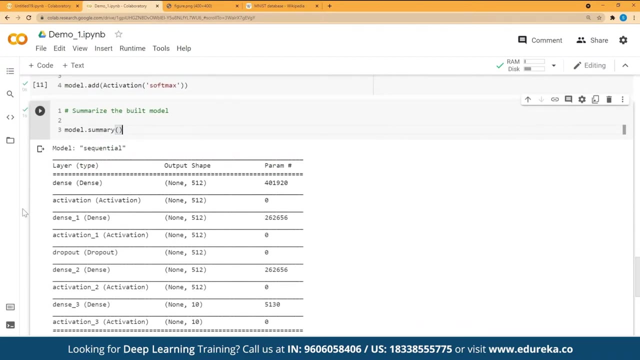 neural network. after the end layer of tense, we are going to again apply a activation function, softmax. okay, and if you want to understand the model you have developed, you can use model dot summary. it will give you what kind of model you have developed. okay, what kind of model you have done. 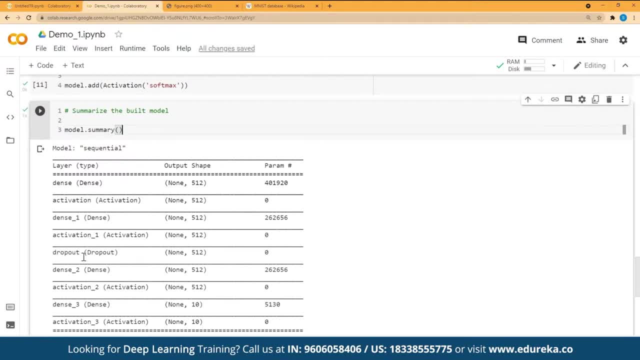 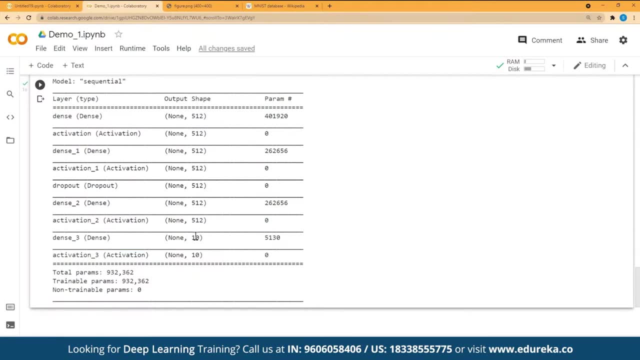 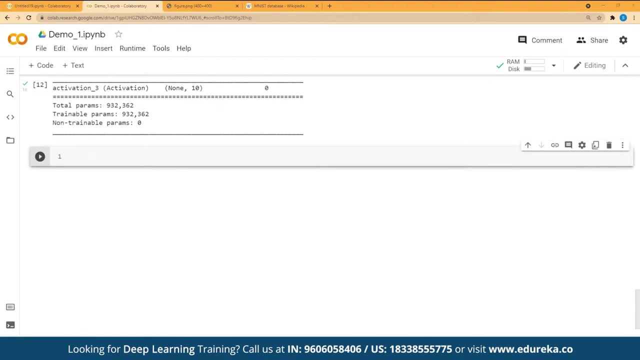 okay, so if you see, this is two dense layers, one and 512, and then we have created a dense layer of output of 10. okay, so we create this. and now what we will do? we will compile the model now. in order to compile it, we need to give some parameters to it. 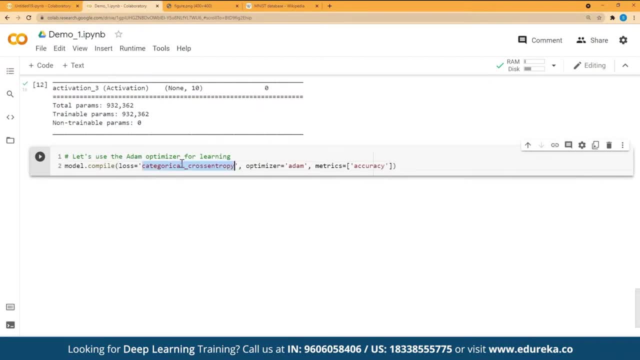 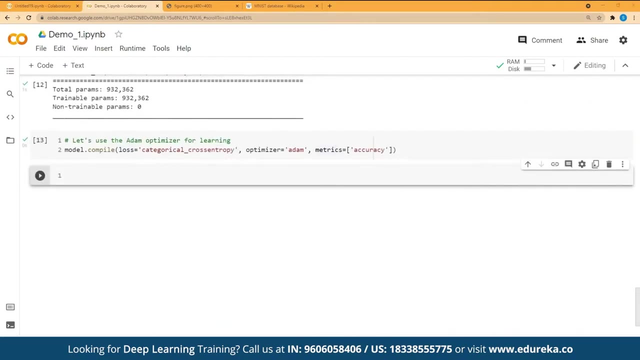 okay, we need to give some important parameters like: what is the loss function, what is the optimizer using, what is the matrix used. so all these needs to be given to the machine, to the neural network. now what i will do, once your model has been compiled, what we will do: we will train the model. so let us train the model. 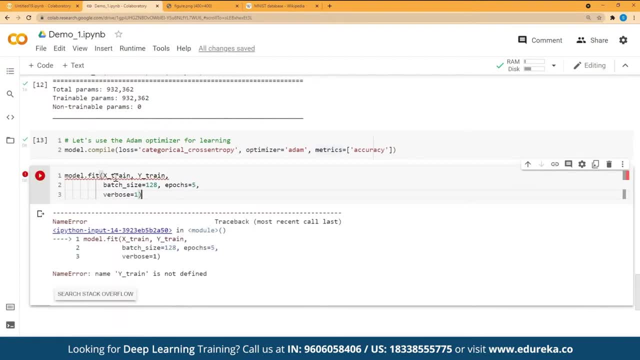 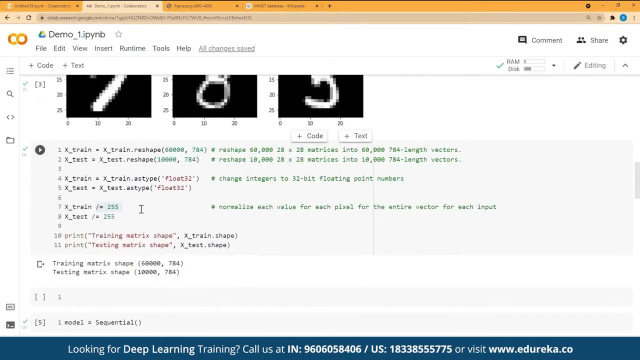 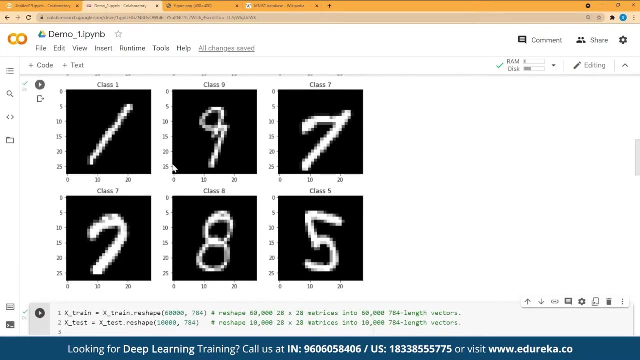 and for training also. we need to pass a few parameters to it, like batch size, epoch, etc. it is saying y train is not defined. let me check. yeah, y train is not defined. so we have not given what is y train. we need to dip, we need to identify that also. okay, it is small y train, if you see. 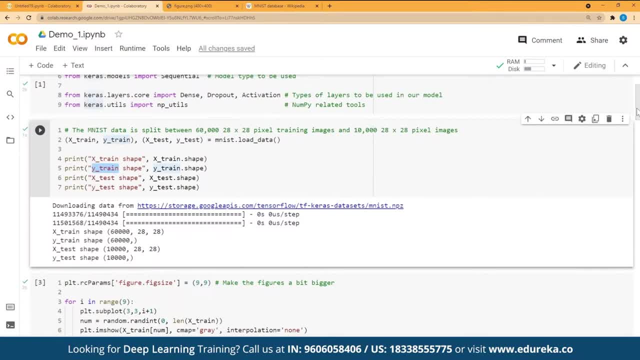 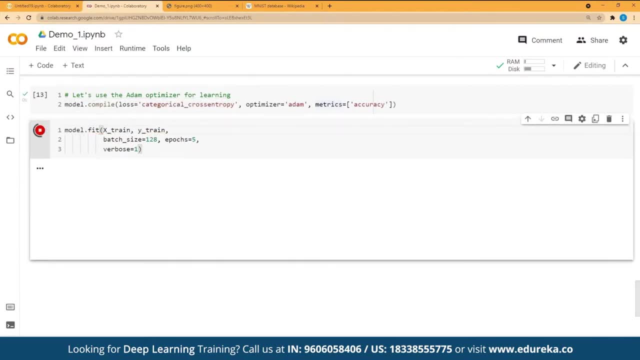 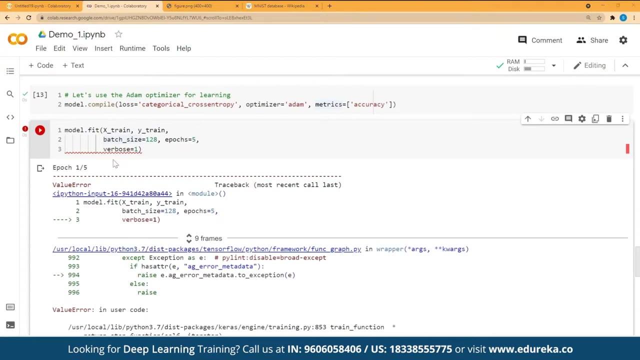 we have defined y train, but we have defined small, small letters y, but here what we have given, we have given capital letters y, so we will reduce it to small and run it again. okay, it is giving us the error. let me just check it, okay. okay, so it seems like there was an issue in the syntax, so it was not giving a. 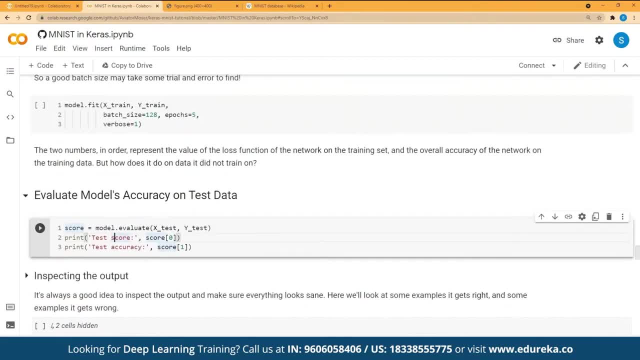 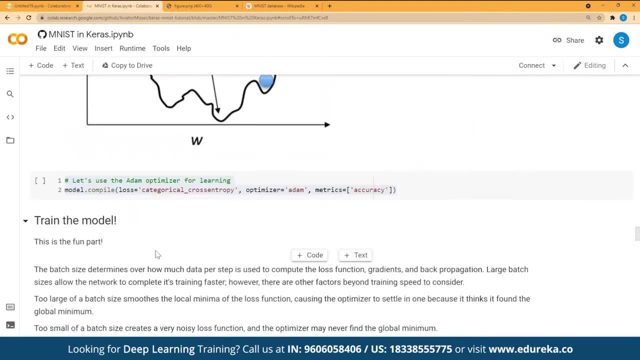 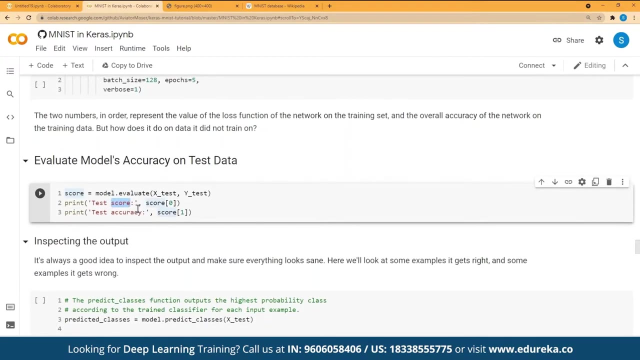 uh, proper result. so, again, i have run it. if you see now, once i run this model, okay, and i check what is the accuracy of this model, it will give me the accuracy of that model and once this model has been trained right, we can use it to predict, with some unknown data, that 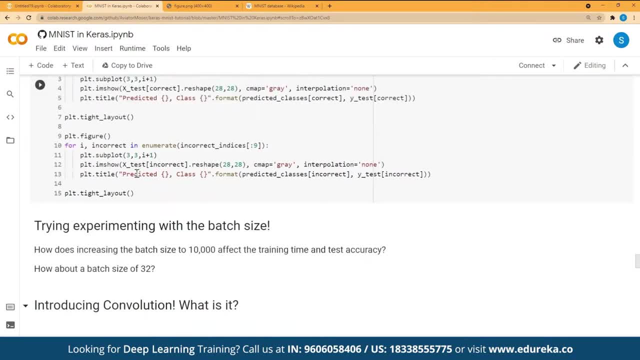 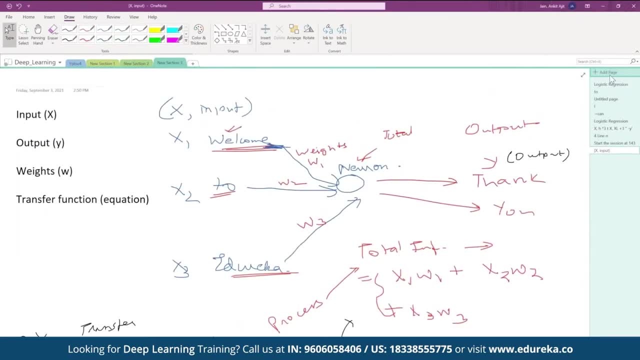 whether it is able to predict it correctly or not. in case it is not able to predict it correctly, what we will do is we will change the number of neurons here. in case your model, in case your model, is not able to train correctly, we will change the number of neurons. 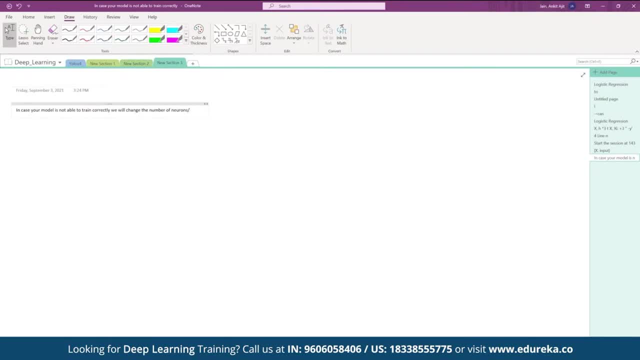 the activation function, the number of layers, right. so all these things you will have to play around so that your model is trained perfectly. that is a very good understanding of your model. it will be a good example to which you learn correctly, and it is giving proper output. What do you mean by proper output? It means 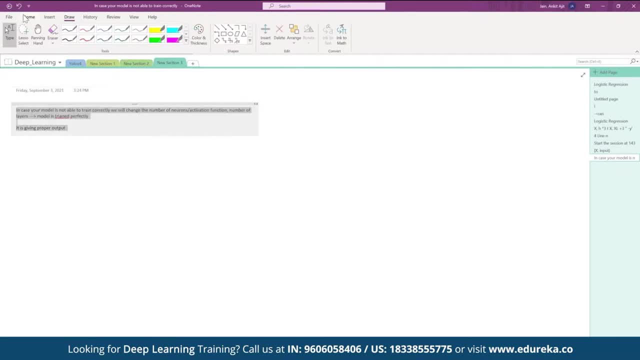 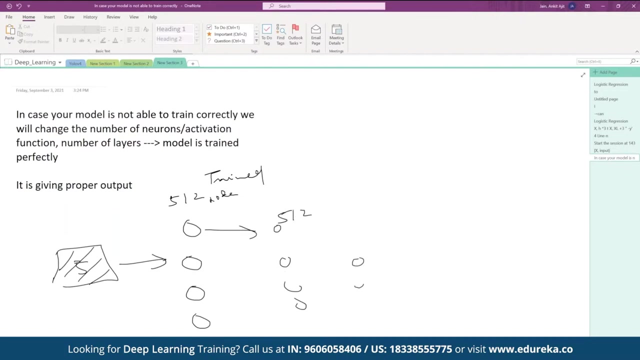 that it is able to identify the images correctly. So suppose you give an input of 5. Okay. Suppose your image is 5. Okay, And now you are giving this to your trained neural network. Just imagine this as 512 nodes. This goes to another layer of 512 nodes, and what it? 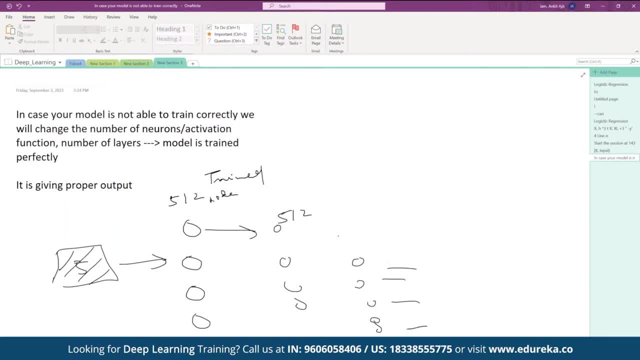 will predict one of the 10 numbers here, Right From 0 to 9.. Suppose it predicts 5,, then your model is well trained, But if it predicts 4,, then your model is not trained. Okay, So then we will change the number of neurons, number of activation functions, number of